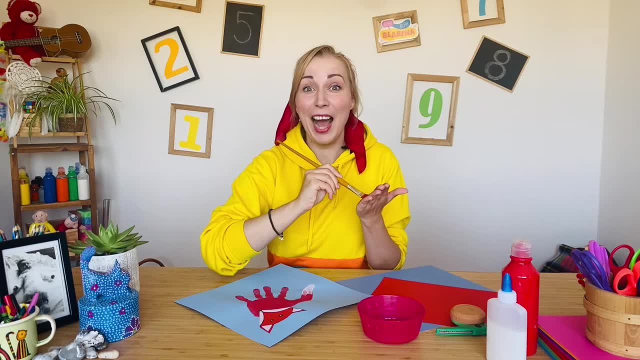 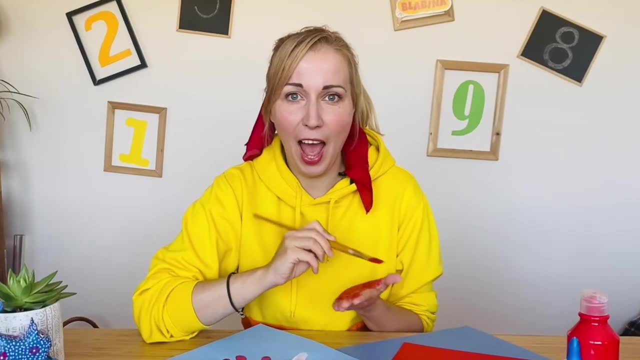 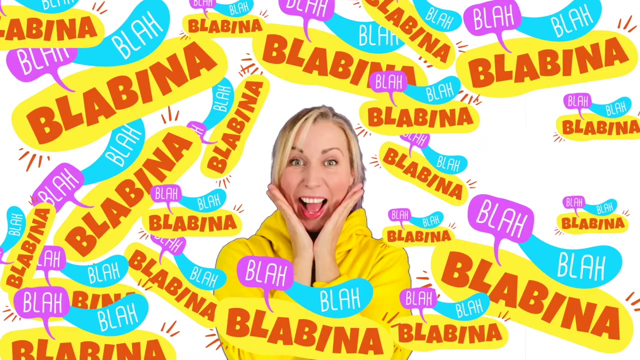 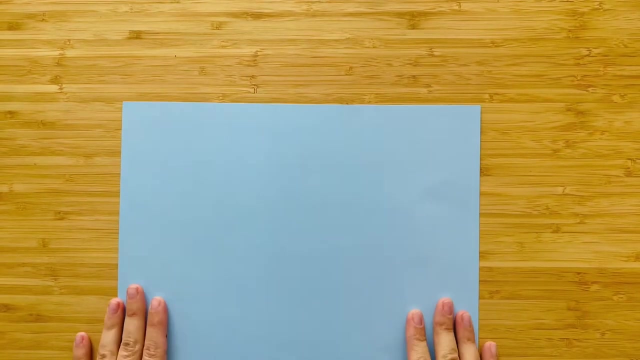 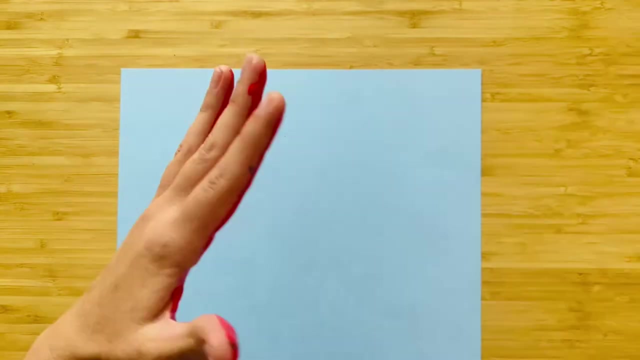 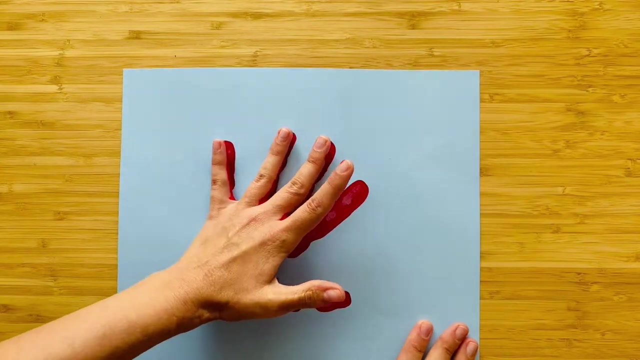 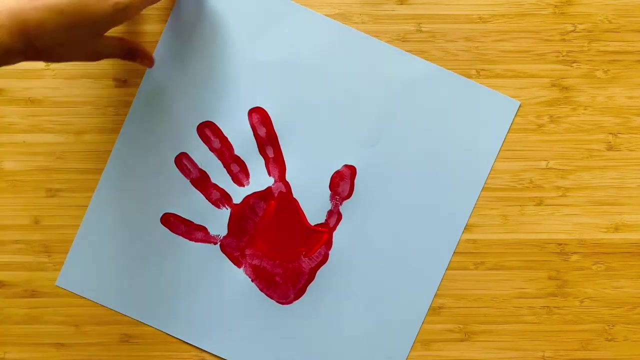 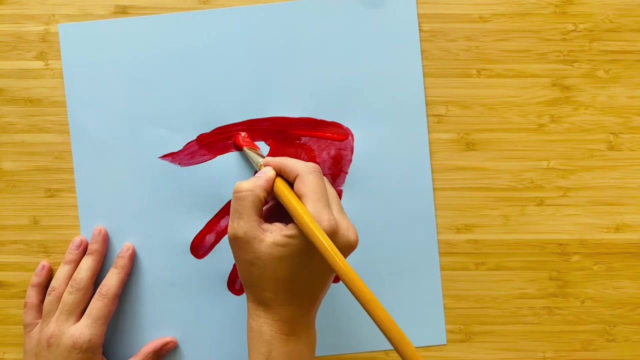 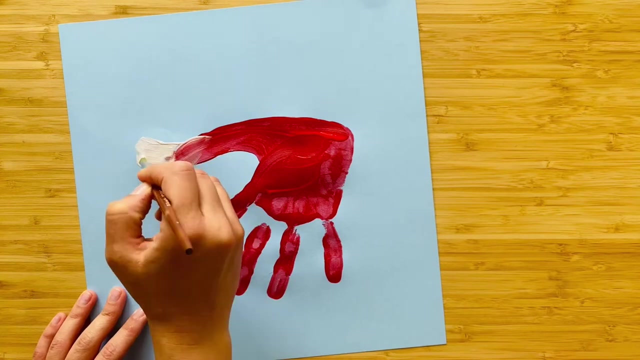 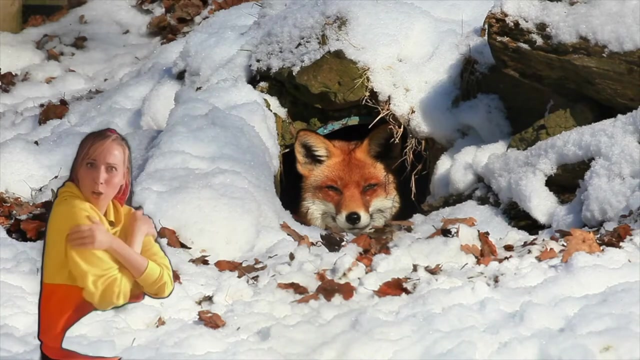 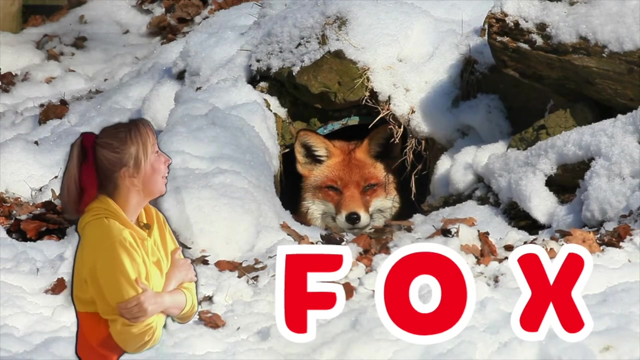 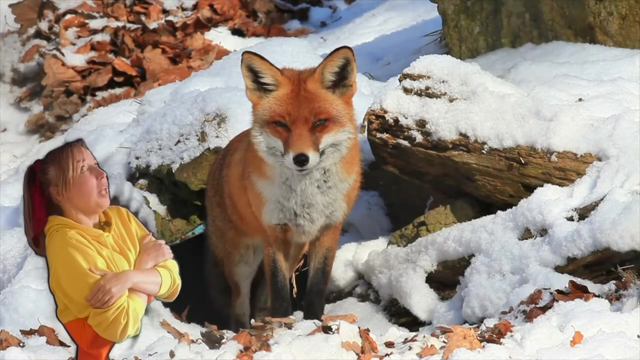 Hi, I am Blabina And today I'm going to make a fox. Watch out for a real fox. Blabla, Blabina, It's cold. Where's the fox? F-O-X fox- Where There's the fox. Hello. 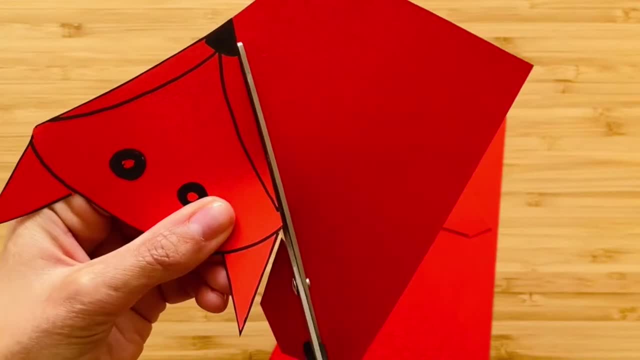 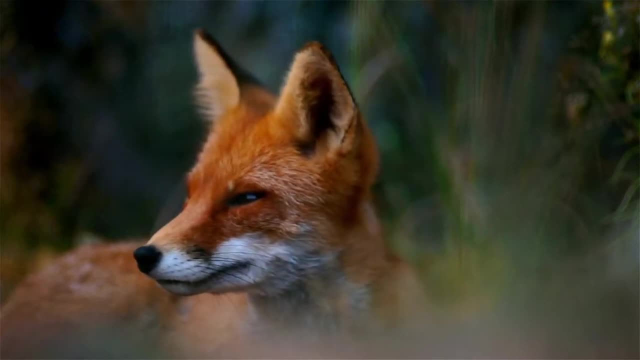 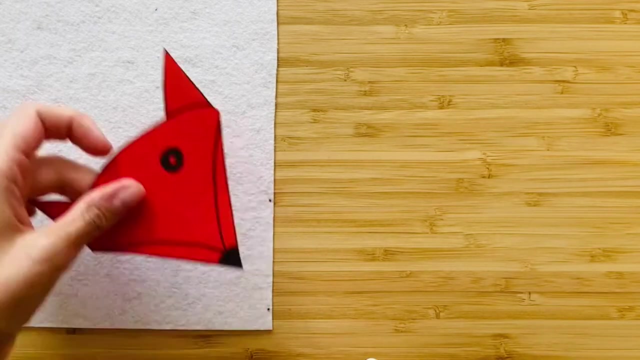 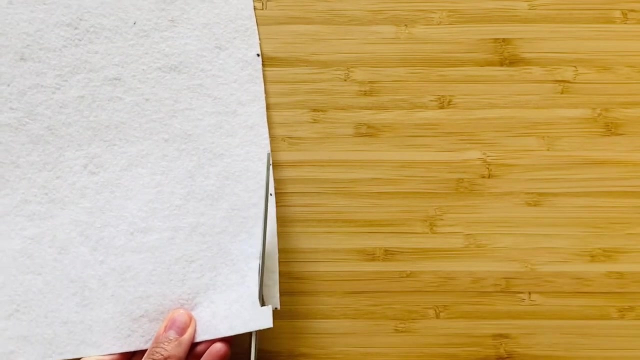 How are you? Foxes have amazing hearing, eyesight and sense of smell. How are you Good? So, how are you Good? Hi, I'm Blabina. Hello, I'm Blabina. How are you Good? 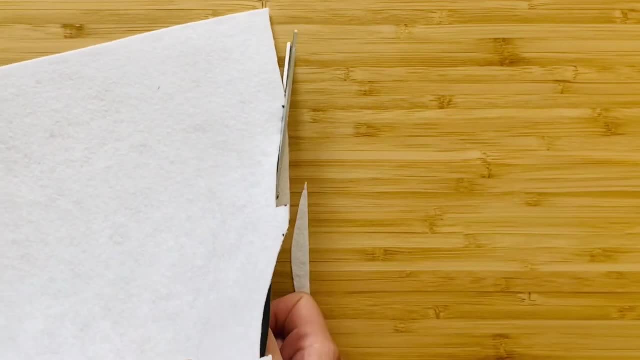 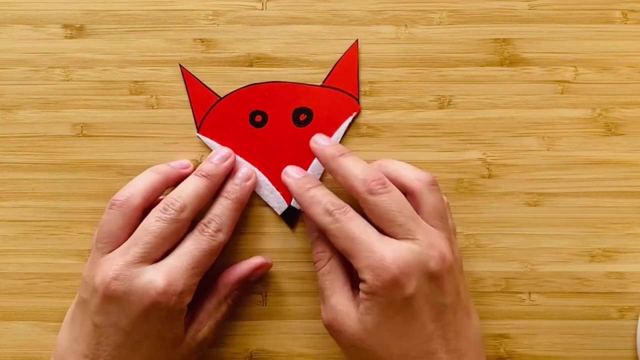 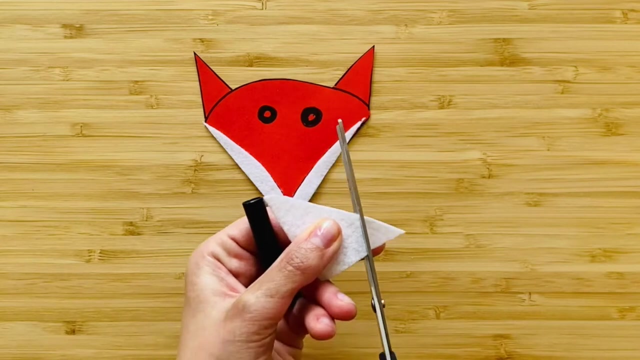 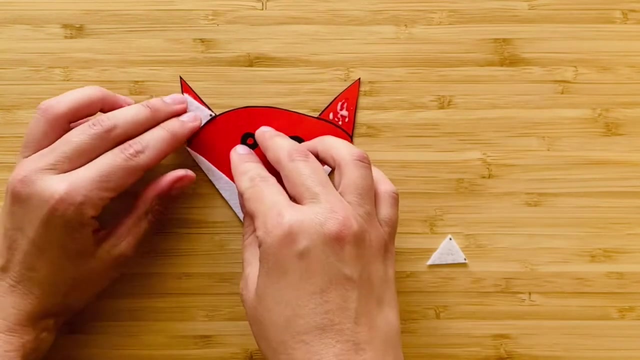 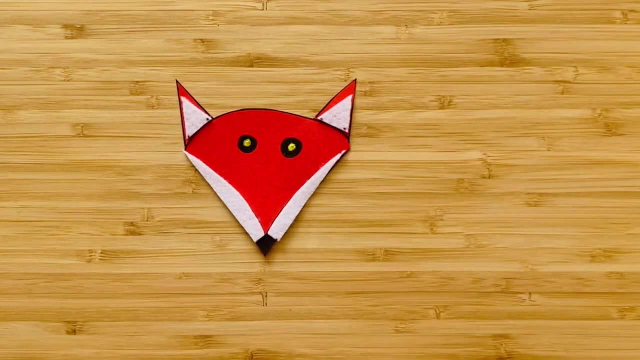 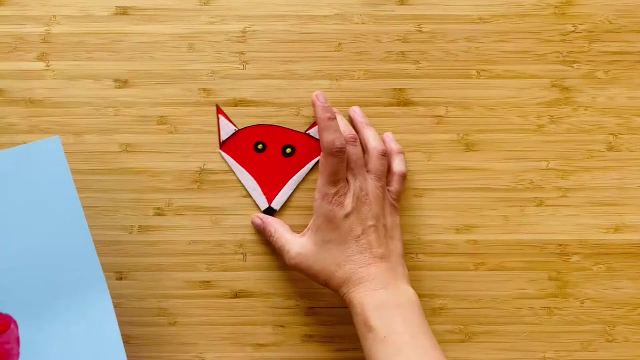 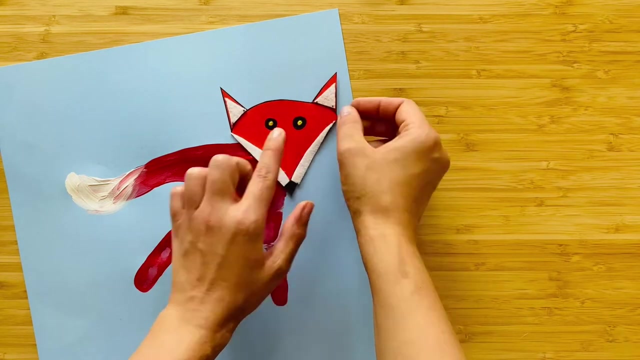 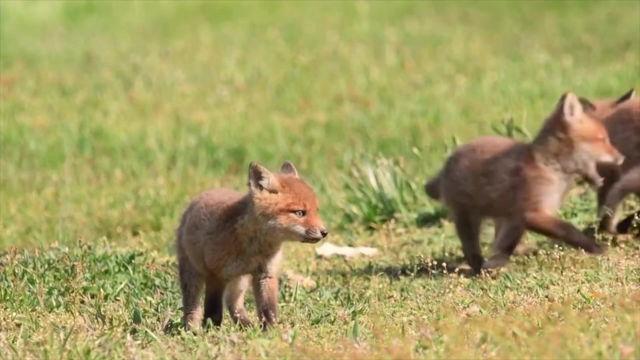 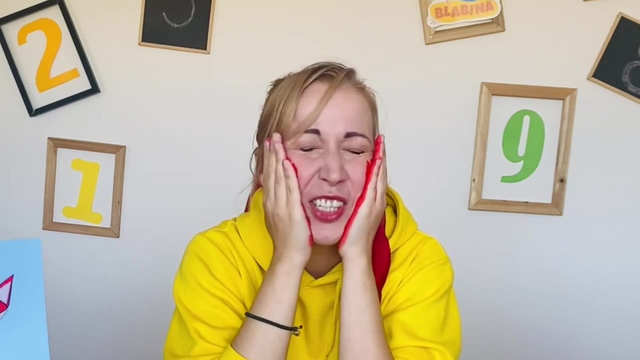 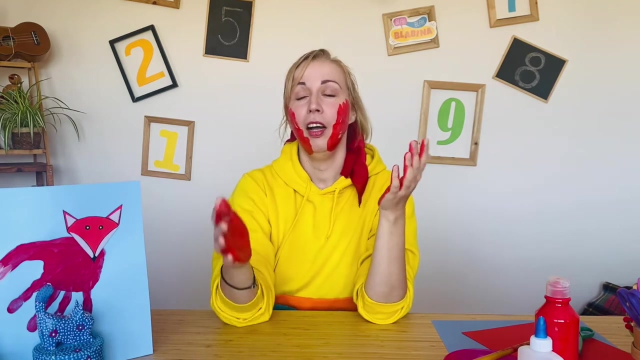 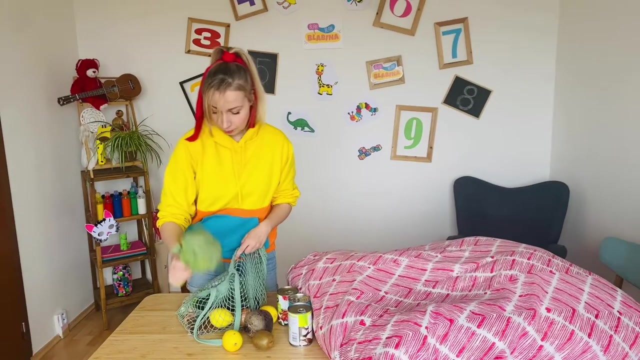 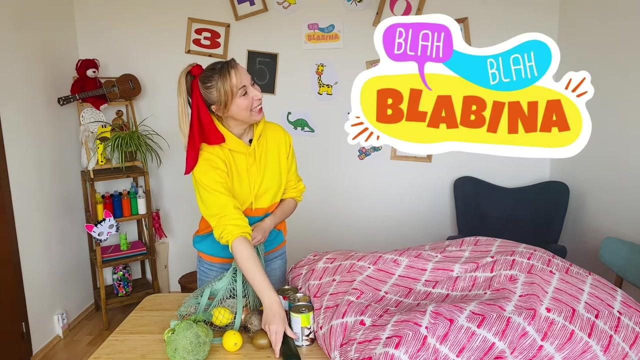 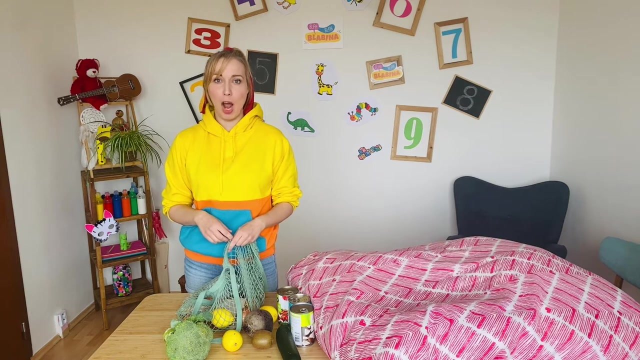 How are you? Good Music, the whiskers on their face and their legs Help them navigate through the dark. GGC, the real fox, So cute. Now, Hi, I am Blondina. It's getting colder outside. I am preparing for hibernation, just like brown bears. 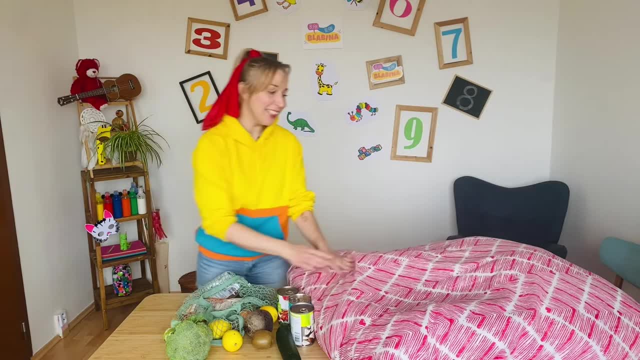 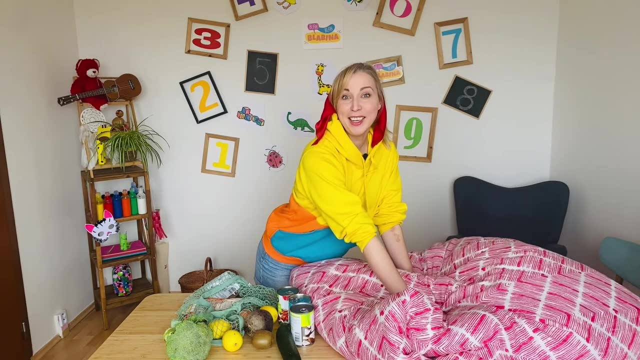 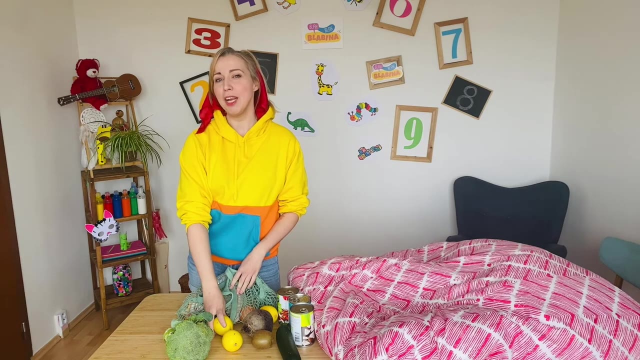 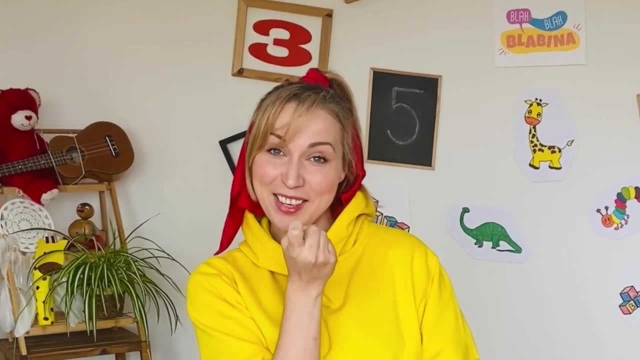 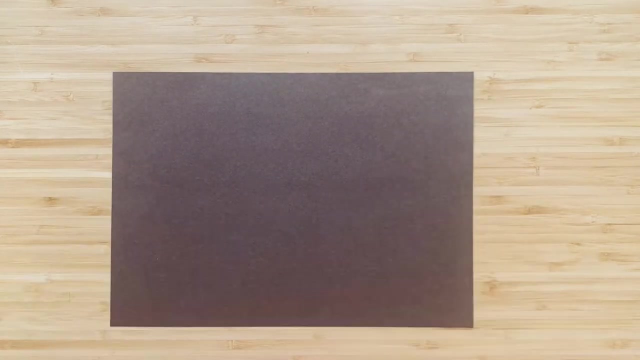 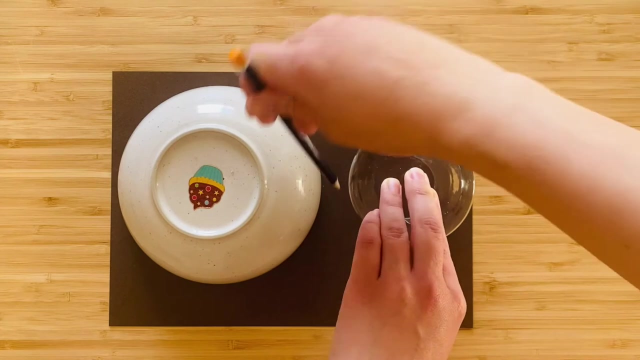 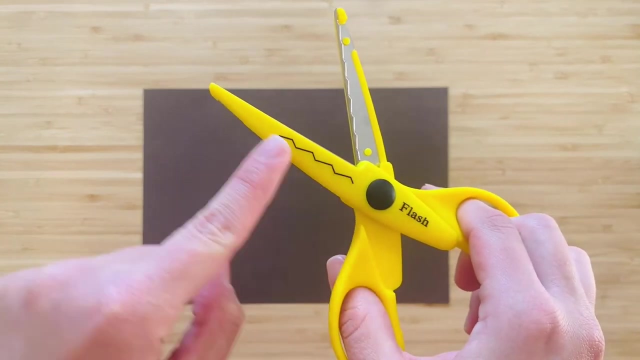 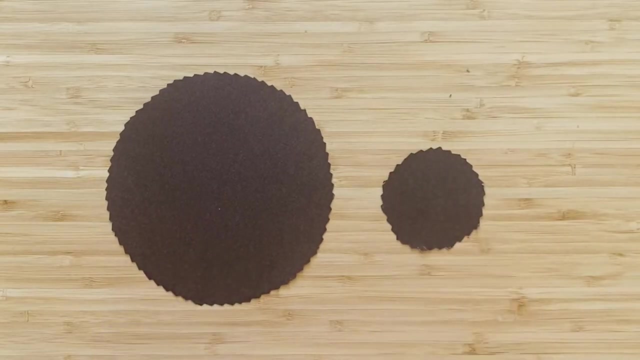 I have plenty of food and my diva to keep me warm and cozy during winter. Do you know what hibernation is? I'll tell you. Blah, blah, blah, biba, Blahblabla In winter, when everything is covered with snow. 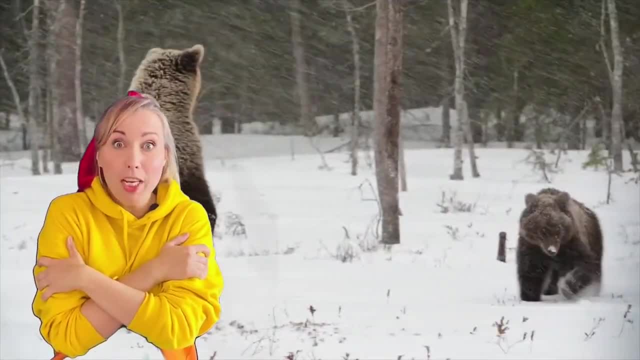 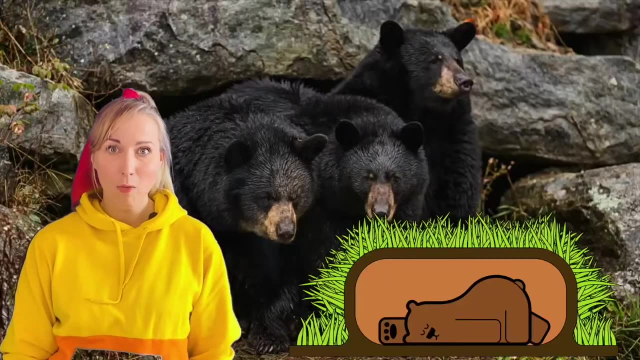 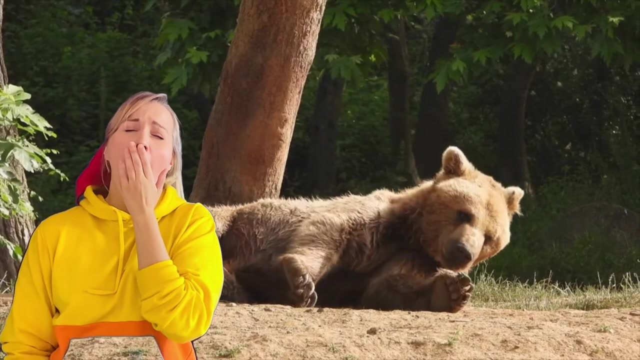 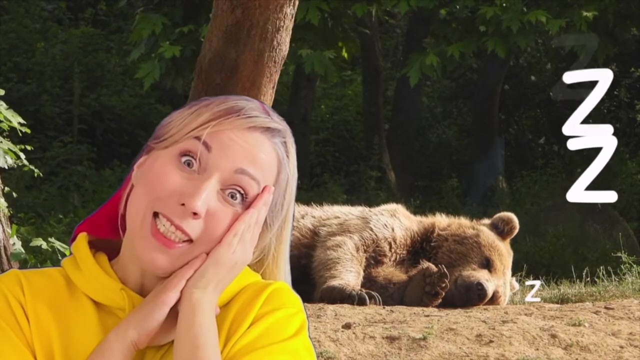 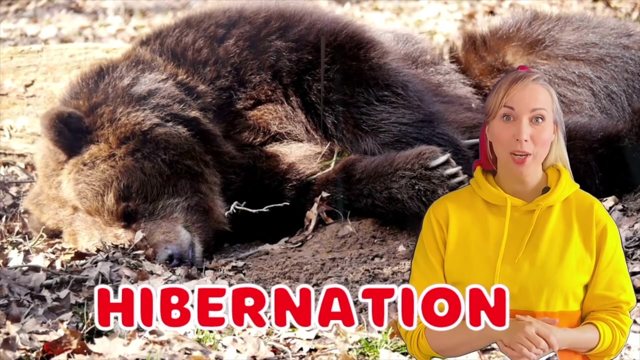 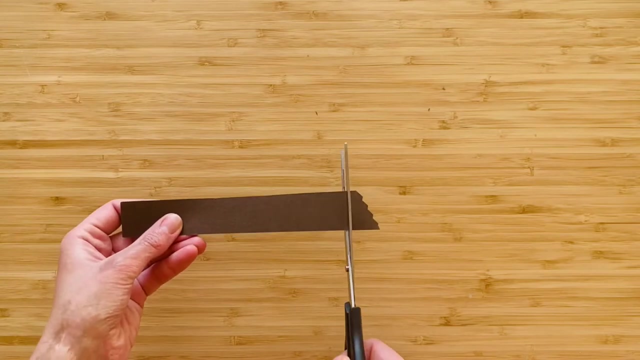 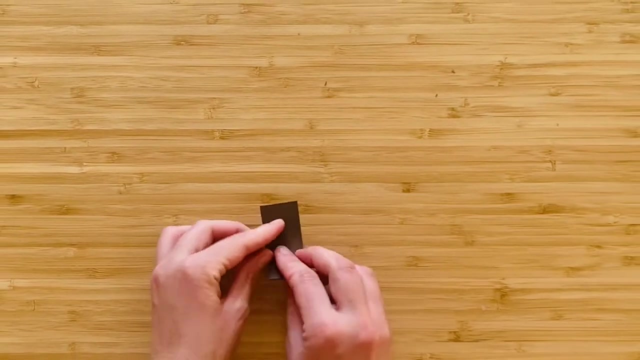 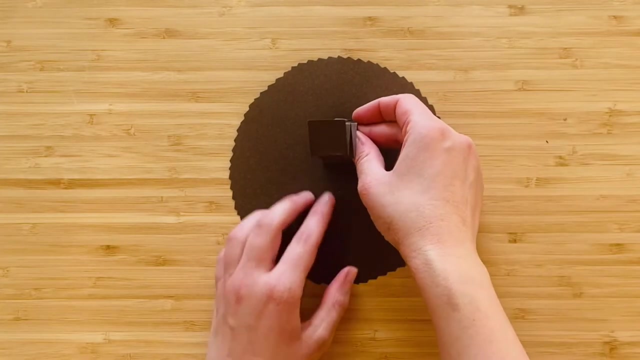 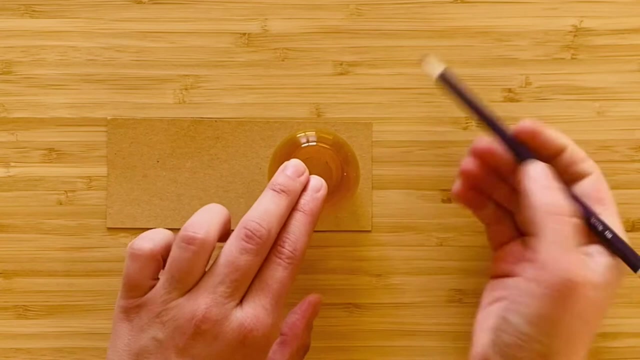 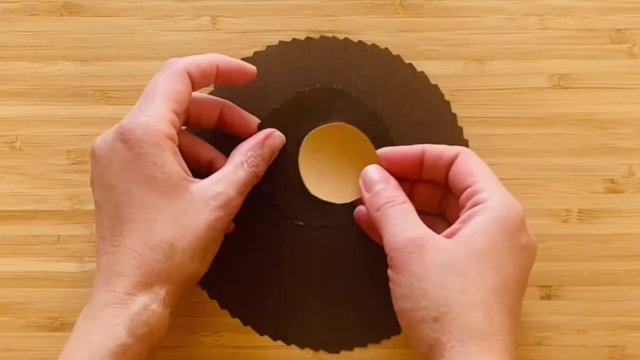 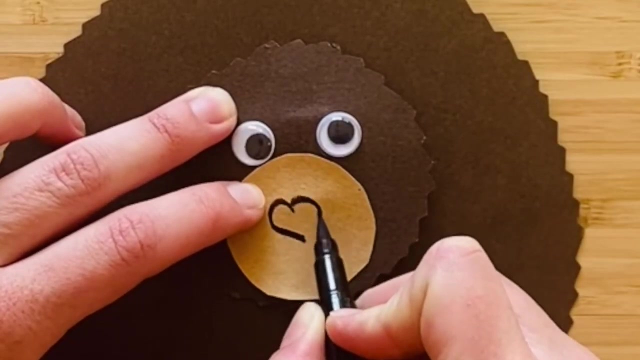 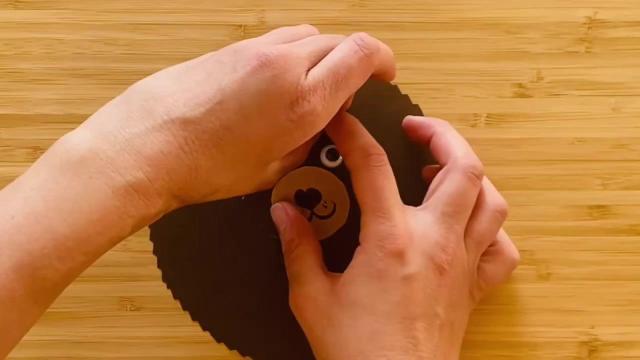 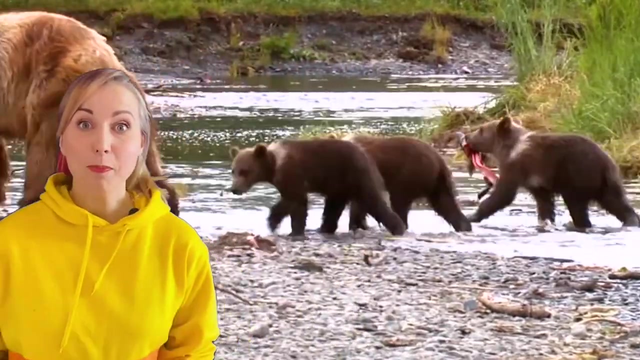 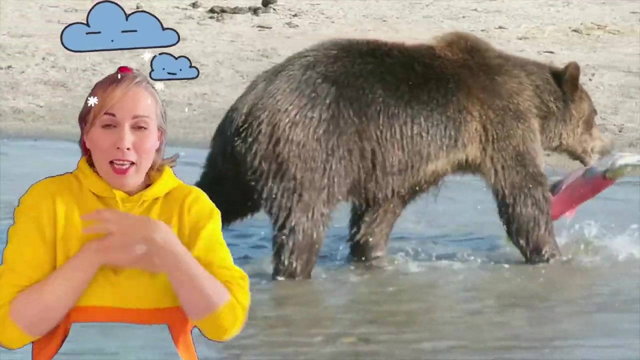 and all the food is frozen. Brown bears find safe and warm place and go into a deep, deep sleep. Sometimes they sleep all winter. This is known as hibernation. This is known as hibernation. What they do is just before it gets really, really, really, really, really cold. they eat a huge amount of food. 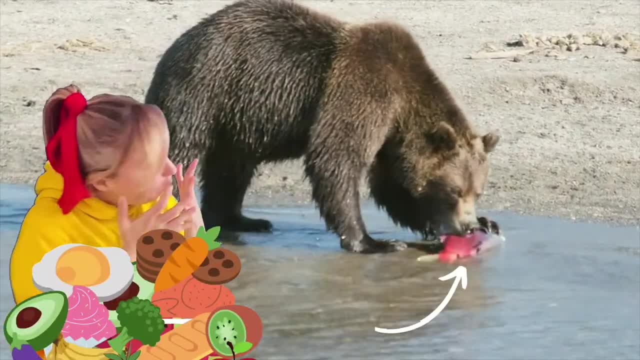 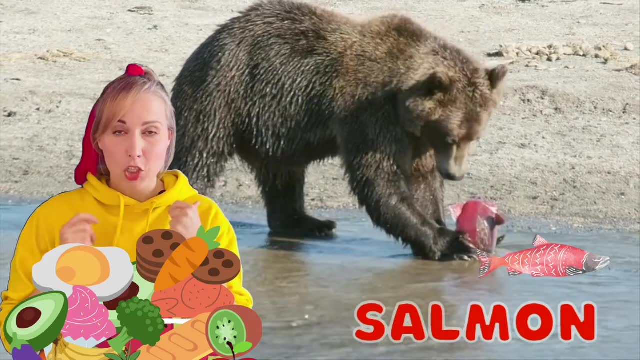 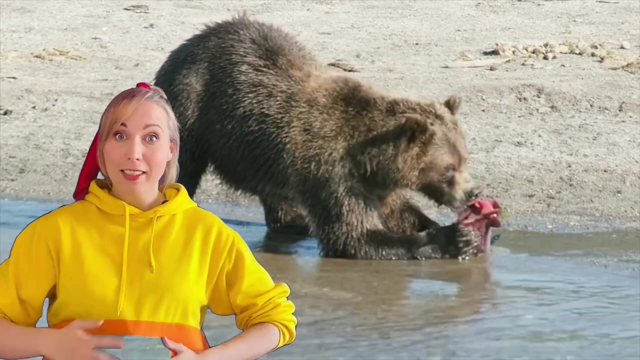 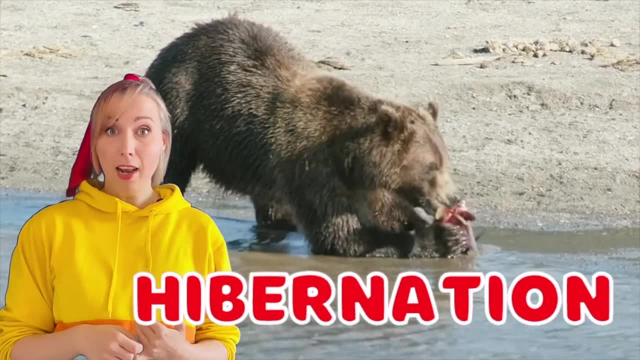 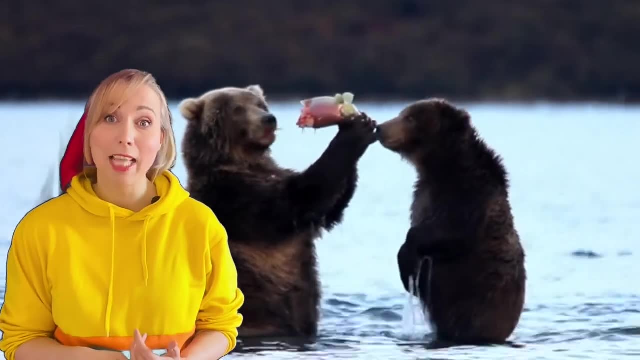 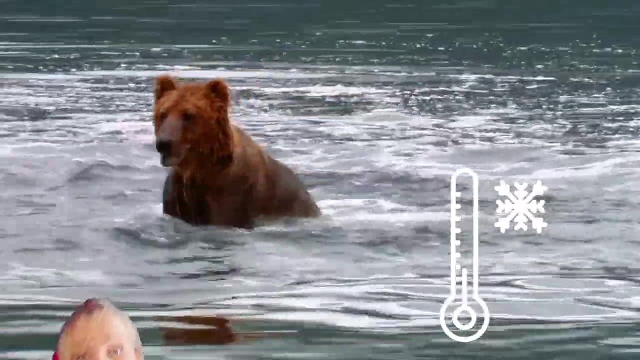 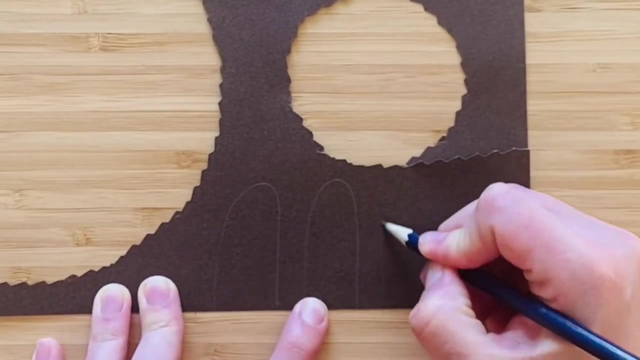 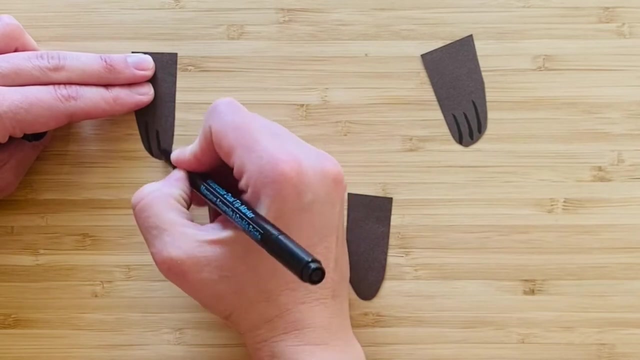 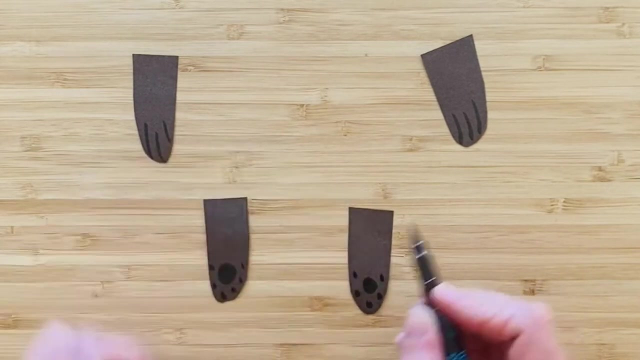 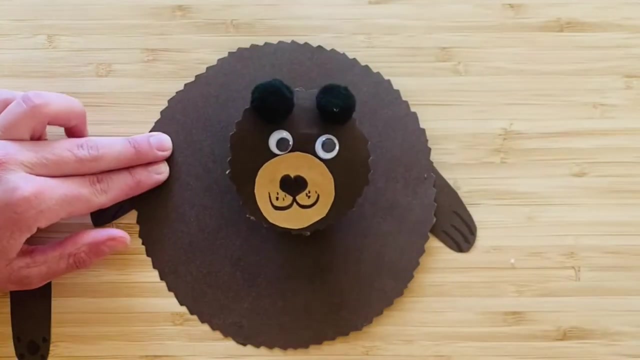 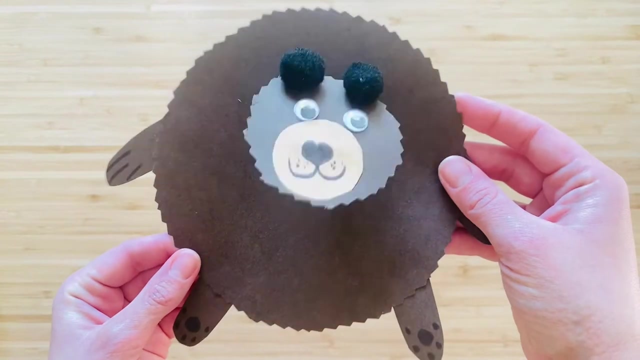 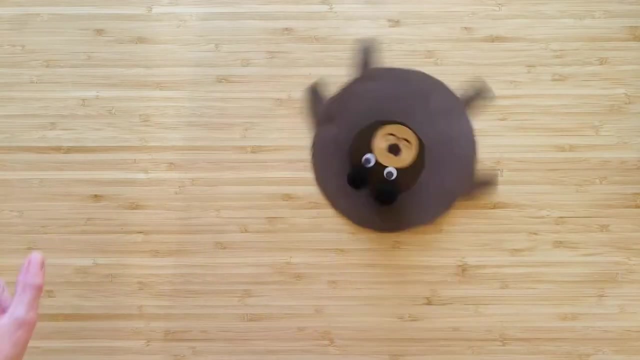 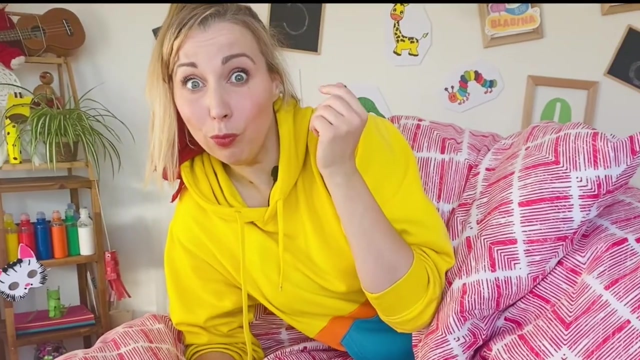 Hibernation helps them stay alive during the cold winter months when all the food is frozen and temperature is low. Hibernation helps them stay alive during the cold winter months when all the food is frozen and temperature is low. Bye, I finished all my food. 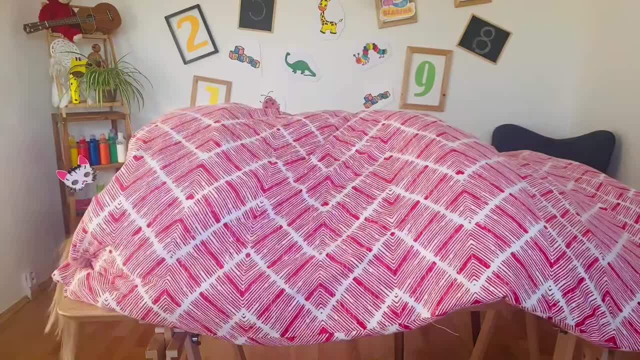 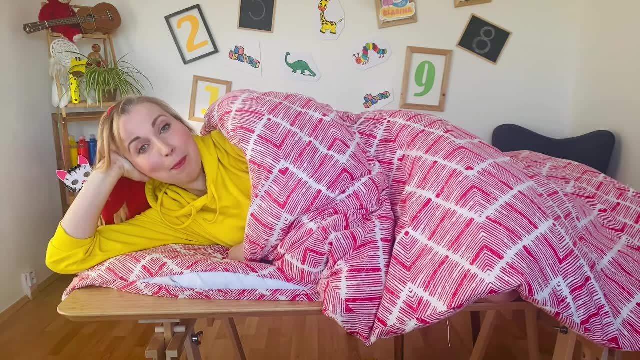 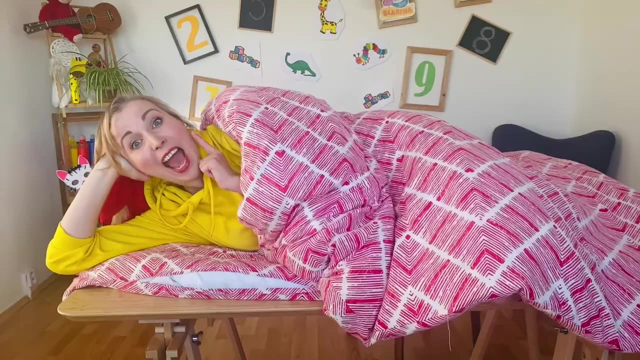 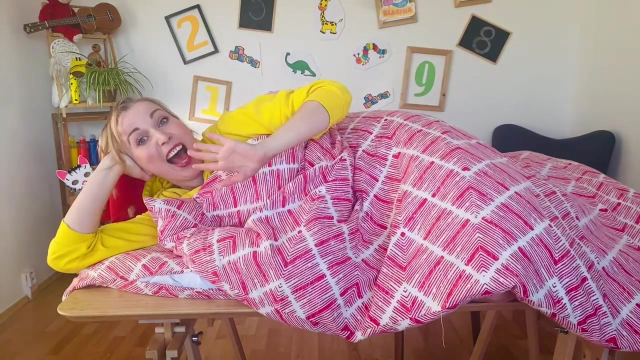 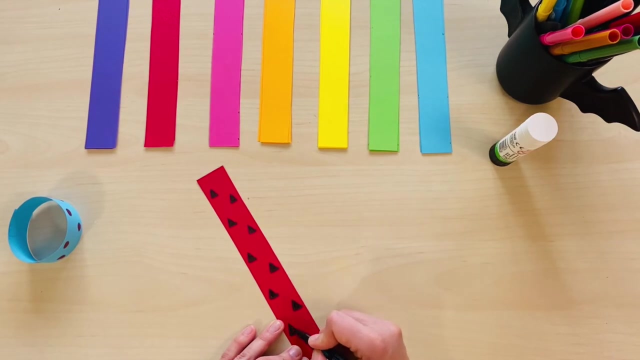 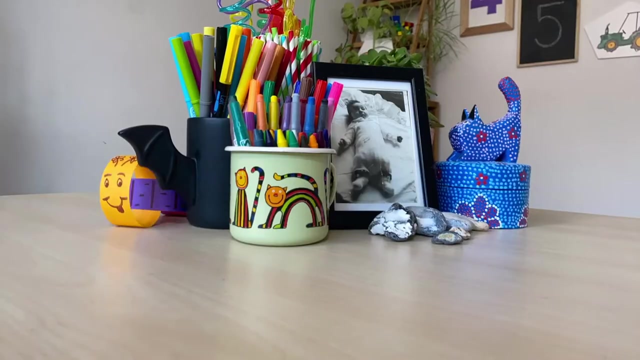 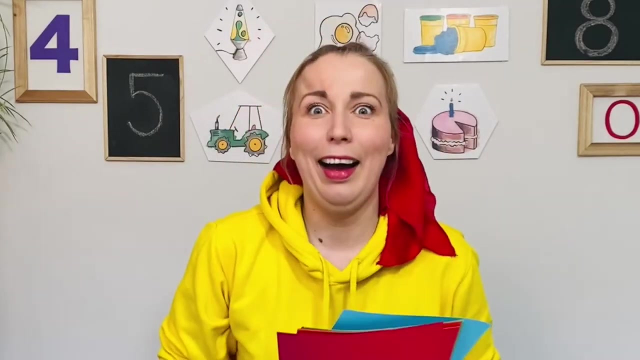 Now let's hibernate, Not yet. It's your turn to make your paper brown bear. Don't forget: you are smart, you are amazing and you can do anything. See you next time. Bye, Blah, blah, blinda. 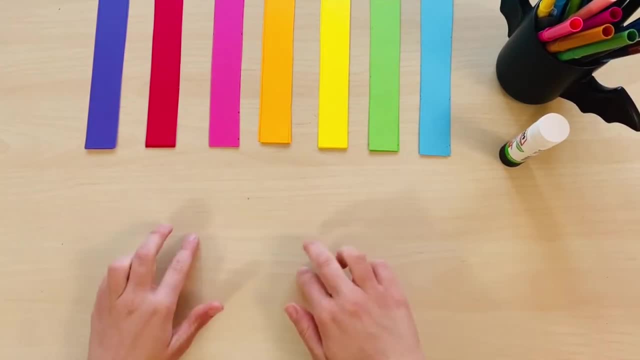 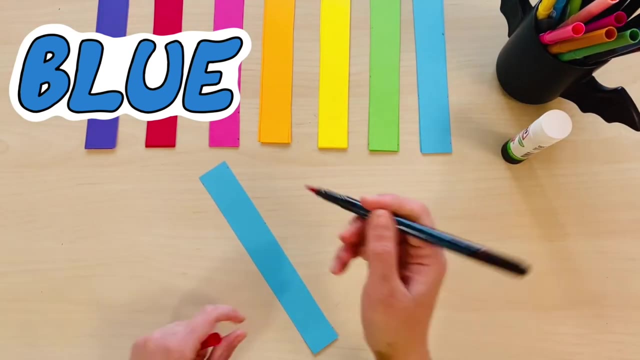 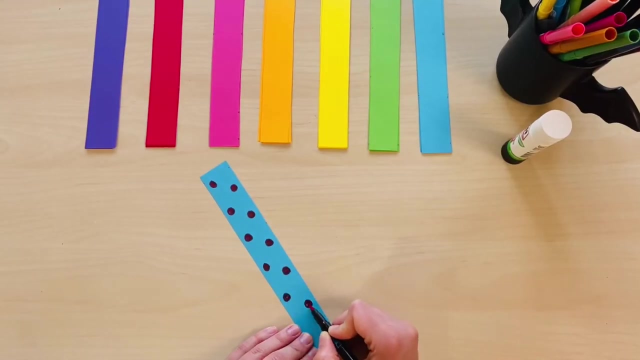 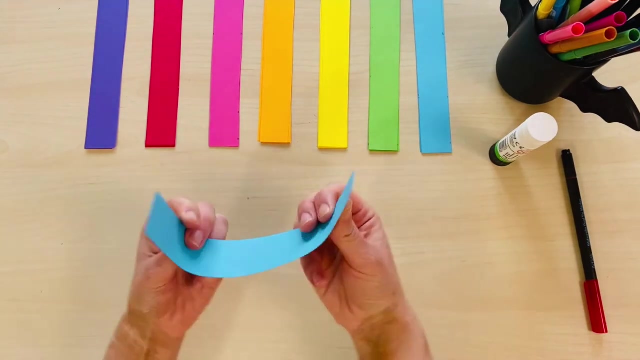 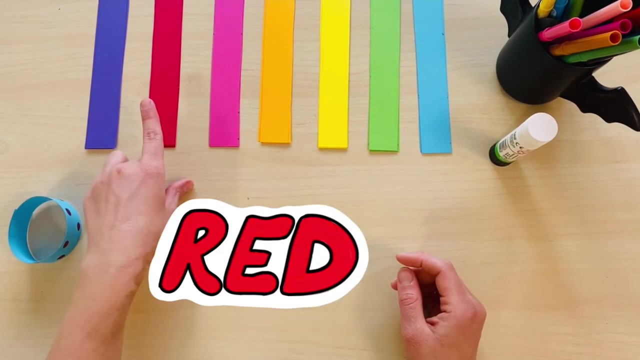 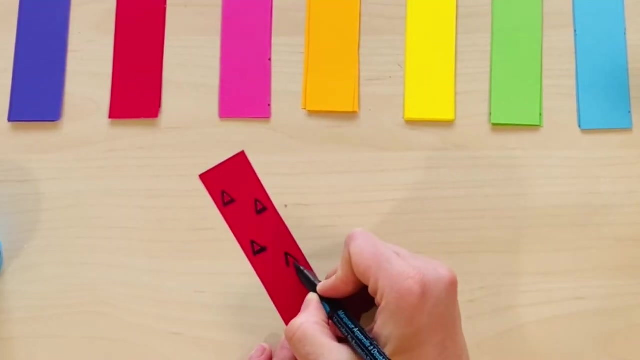 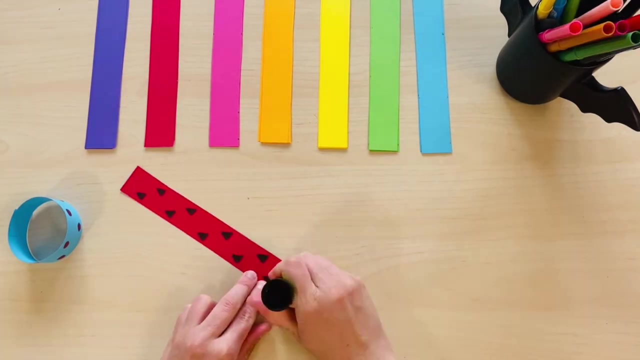 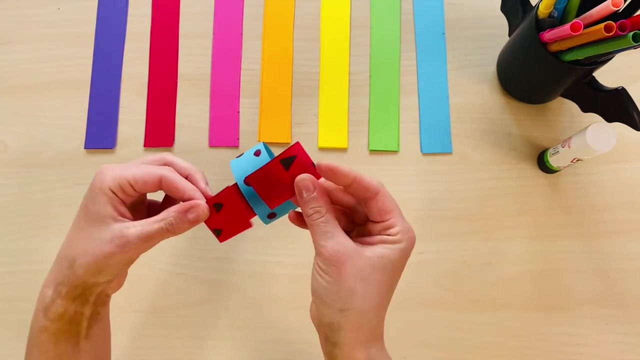 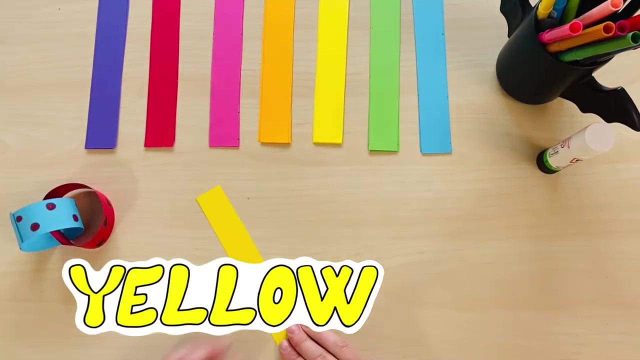 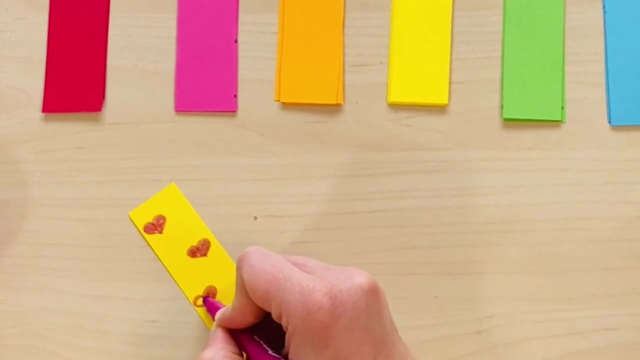 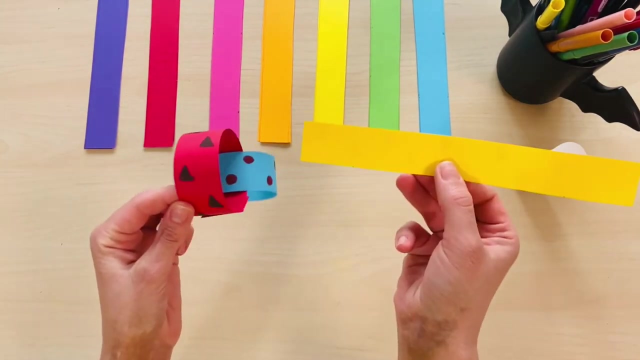 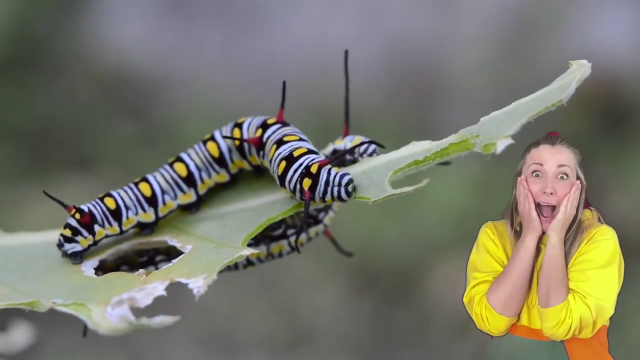 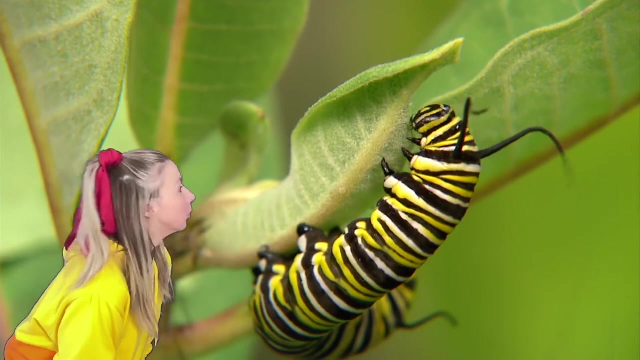 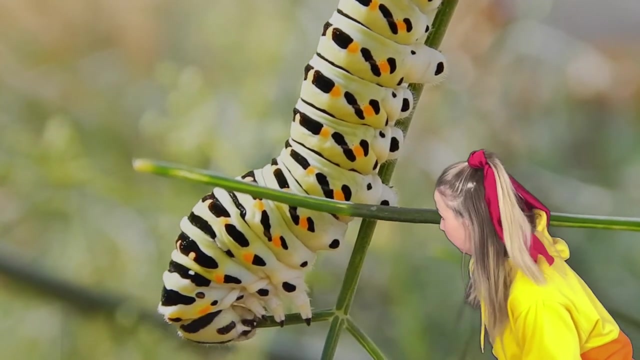 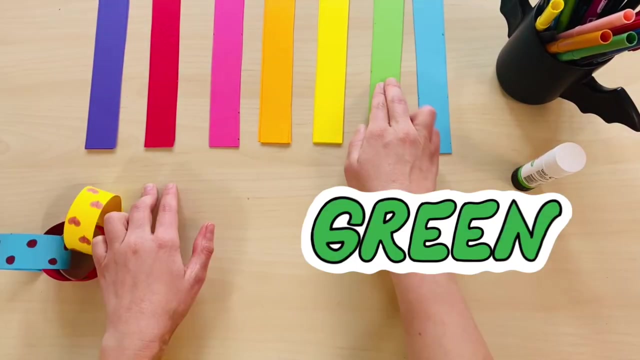 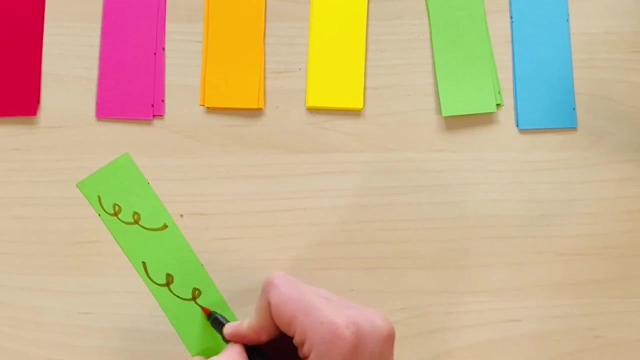 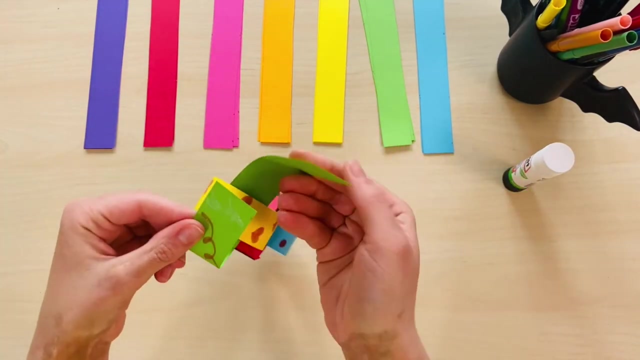 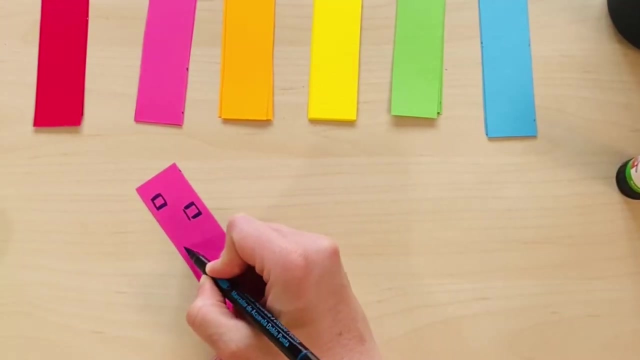 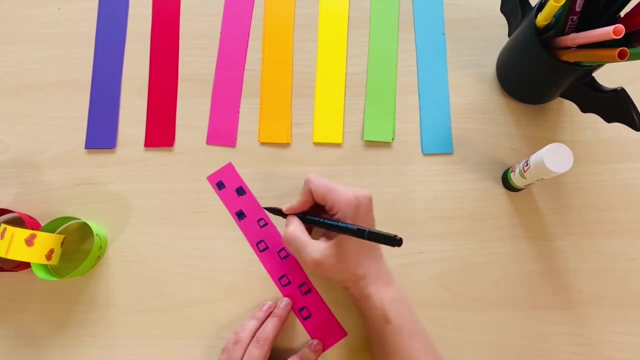 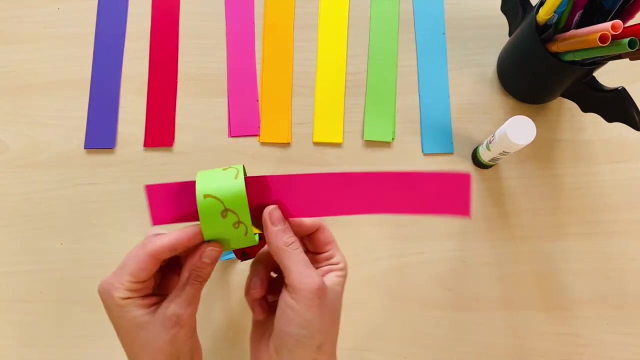 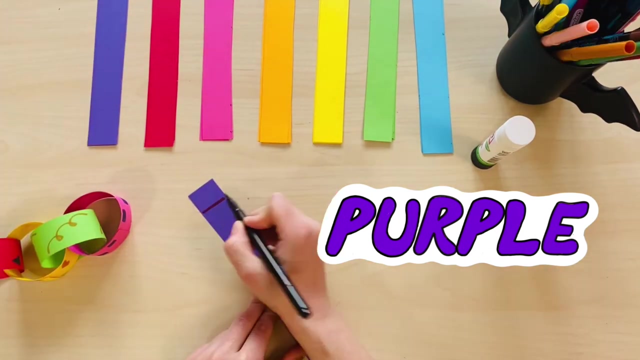 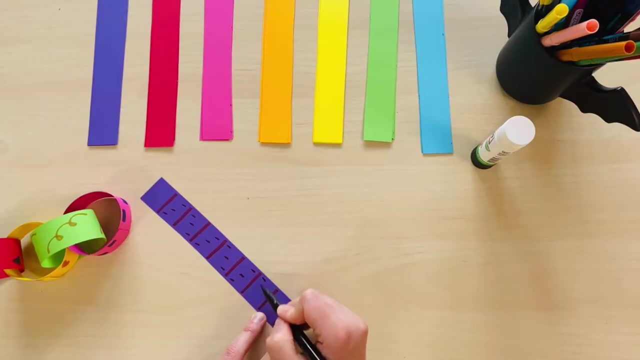 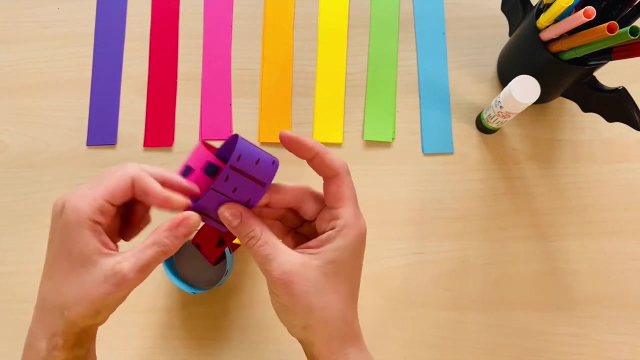 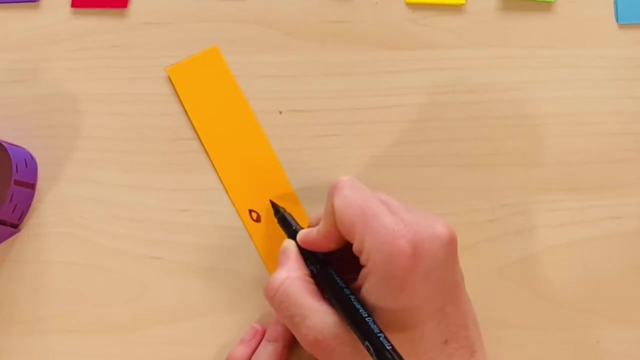 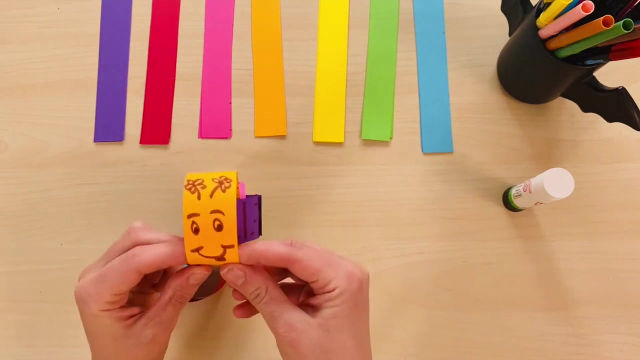 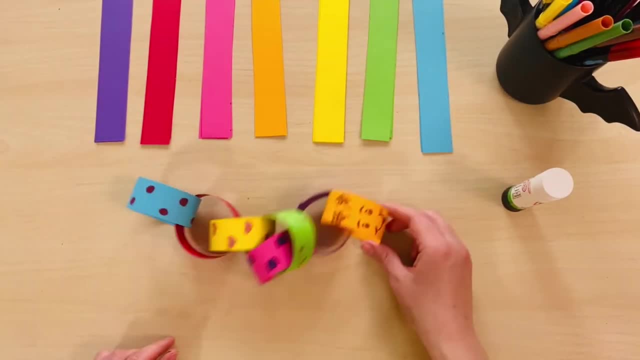 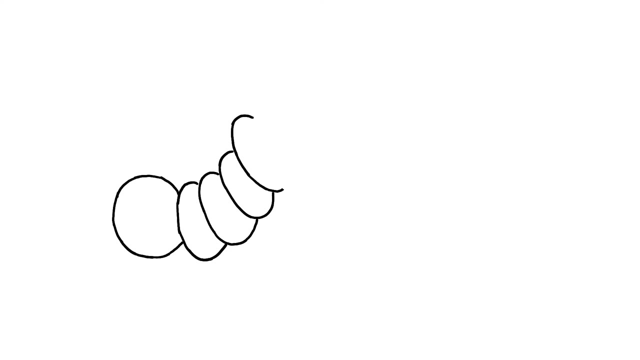 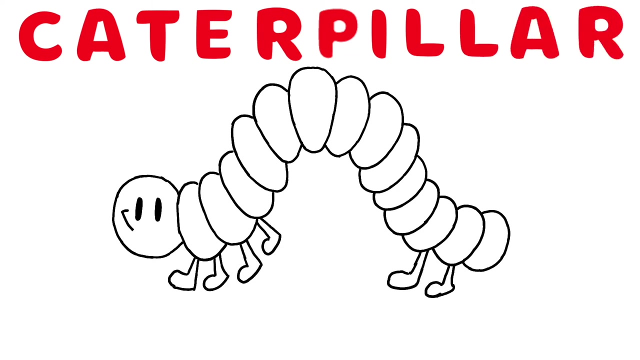 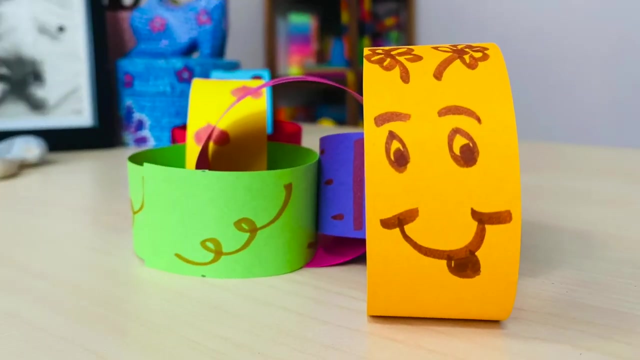 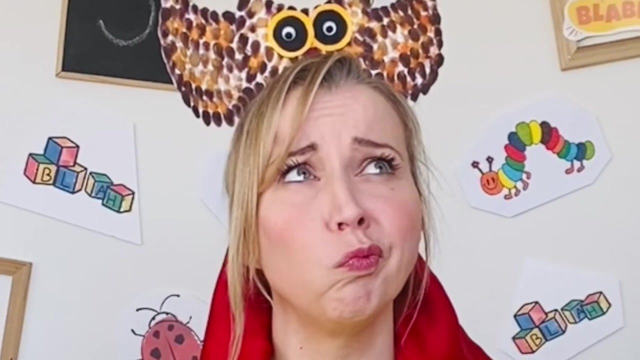 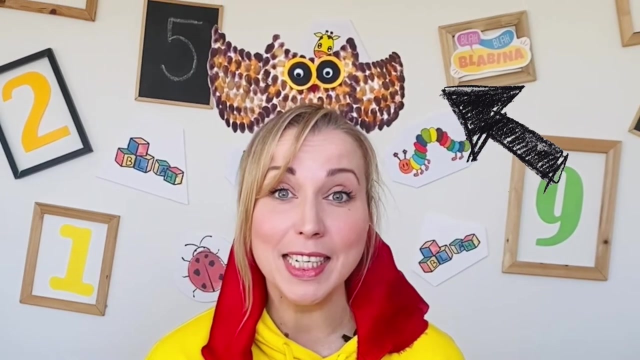 Red, Purple, Green, Yellow, Pink, Yellow, T-A-T-E-R-P-I-L-L-A-R. Caterpillar. You are smart, you are amazing and you can do anything. Is there something on my head? What is it? Caterpillar, Caterpillar. 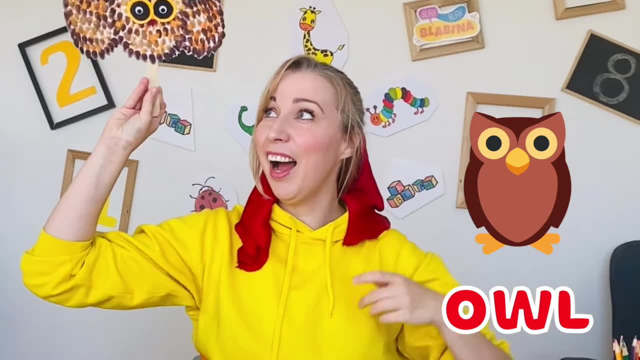 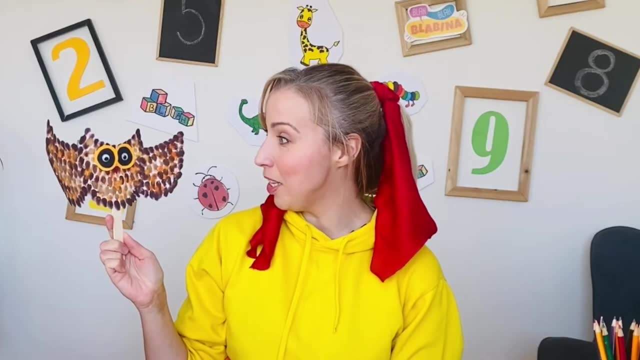 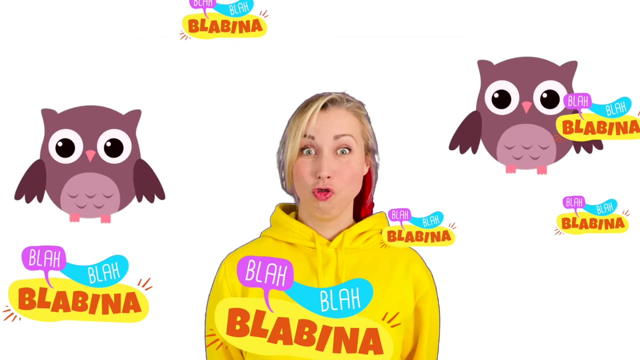 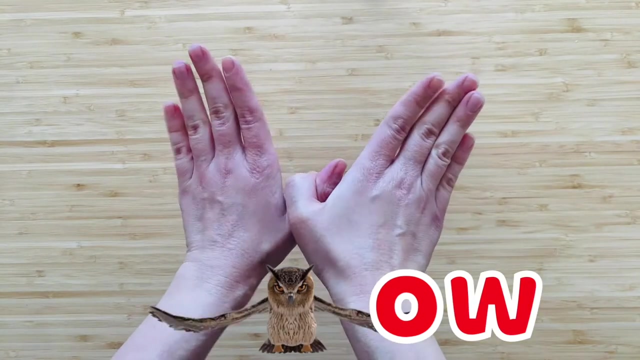 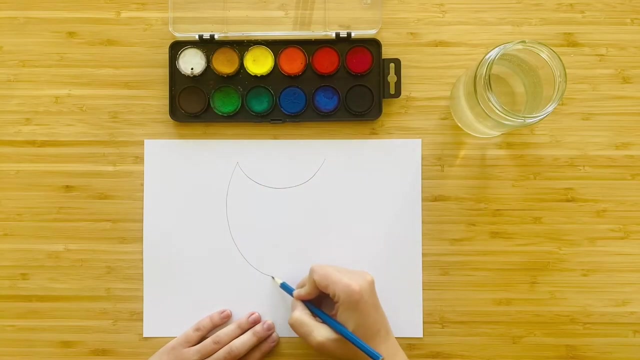 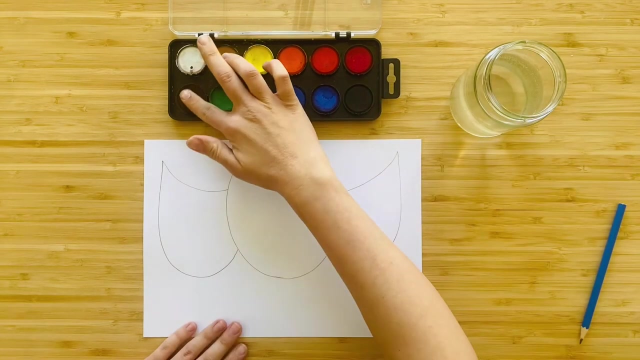 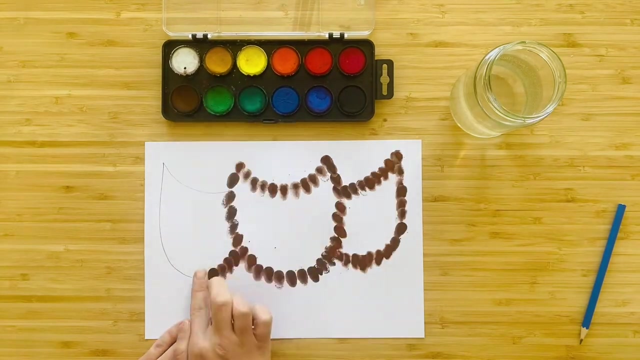 I'm down, It's an owl. Hello, my name is Peter. Nice to meet you, Peter. I'm Blabina Blah blah, Blabina O-W-L. owl O-W-L. What is happening? 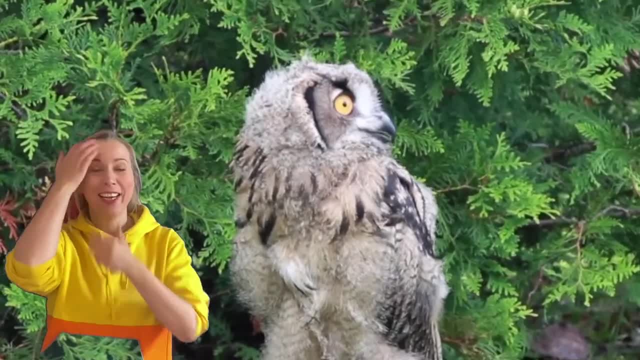 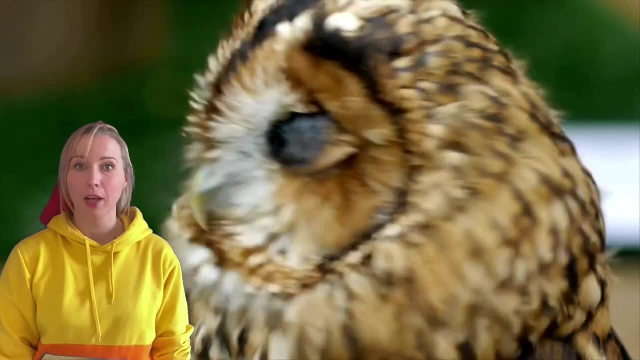 O-W-L owl. O-W-L owl. O-W-L owl. Owl's eyes are set in position O-W-L owl- O-W-L owl- O-W-L owl. They can't move them like we do. 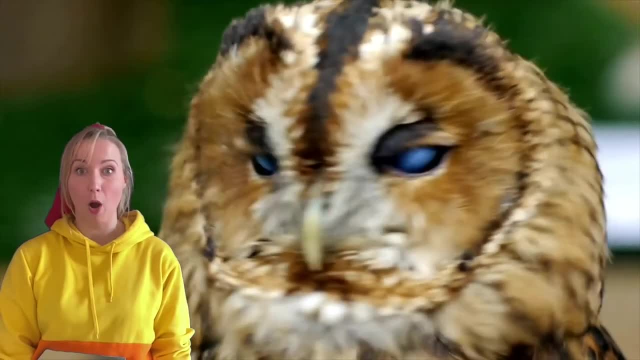 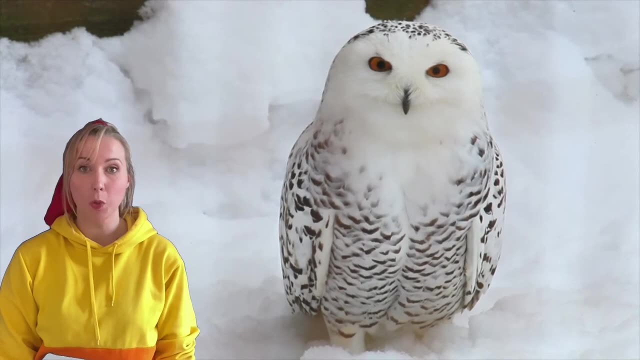 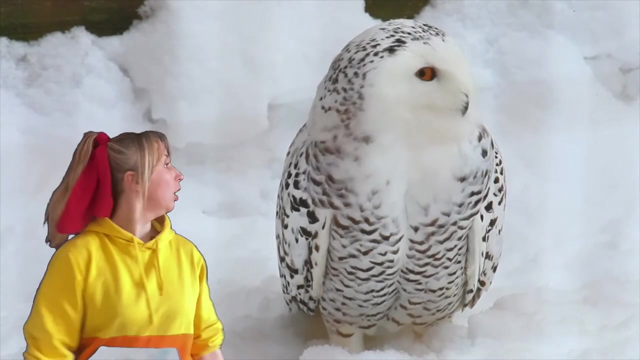 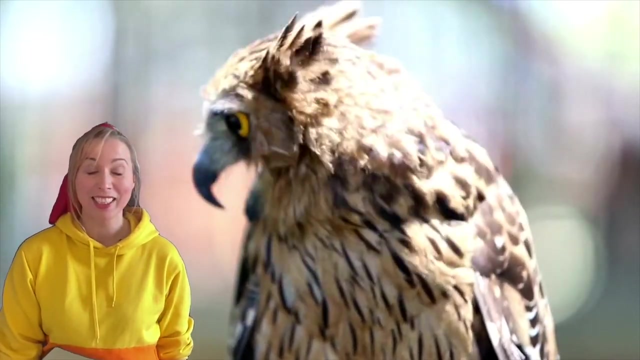 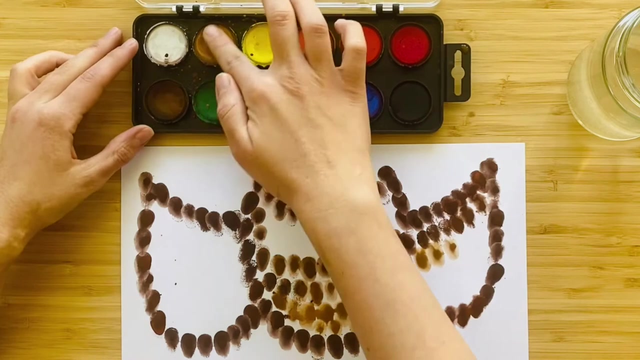 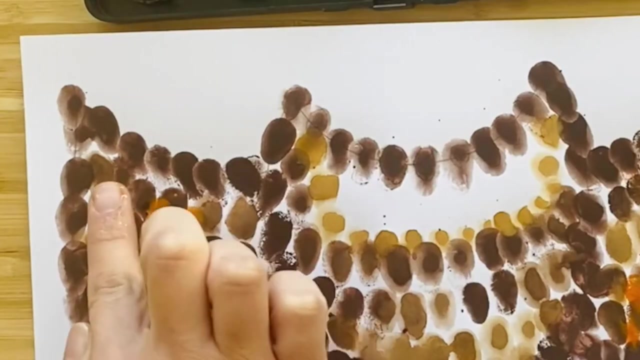 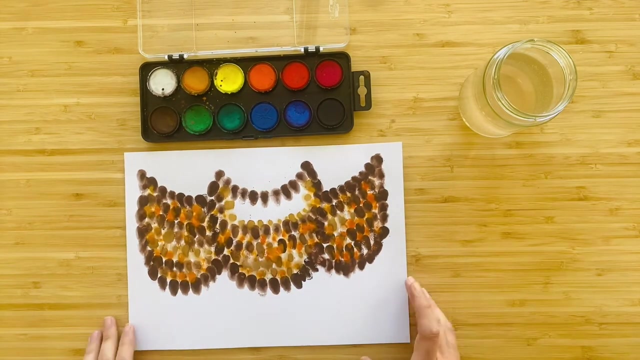 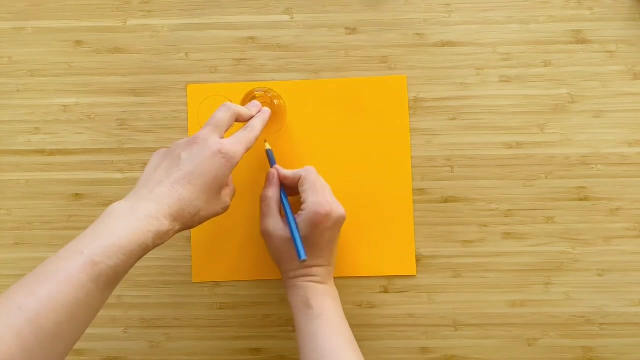 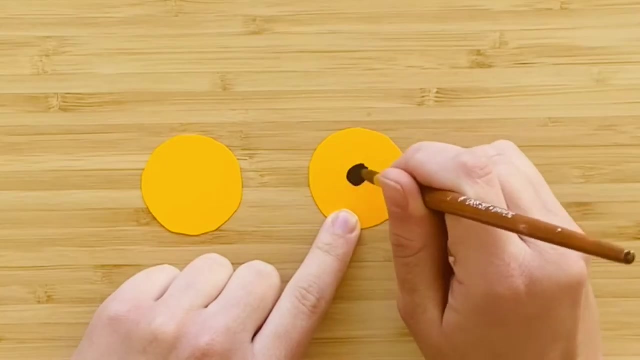 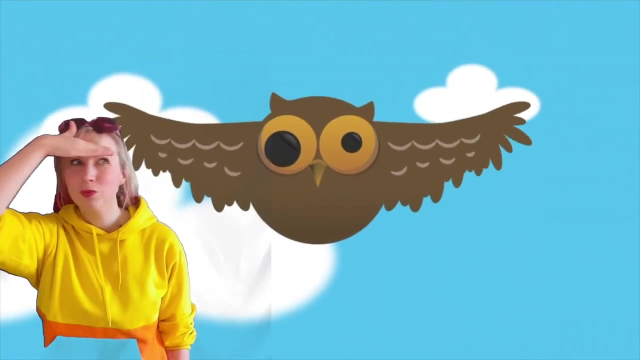 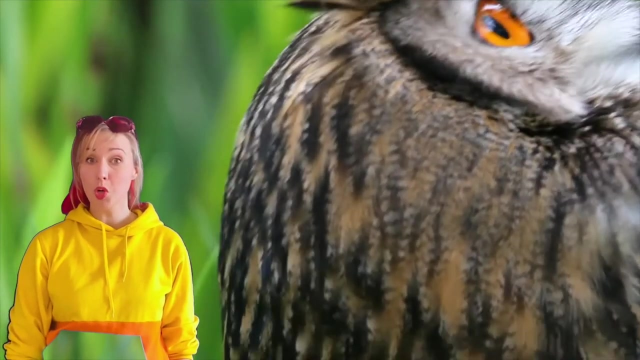 When they want to look around, they have to move their whole head. Their neck can rotate 270 degrees, That's almost all the way around. Am I doing it? Did I do it? Did I do it? Can you try? Oh, Owls are far sighted. that means they can see really, really well, far, far away. 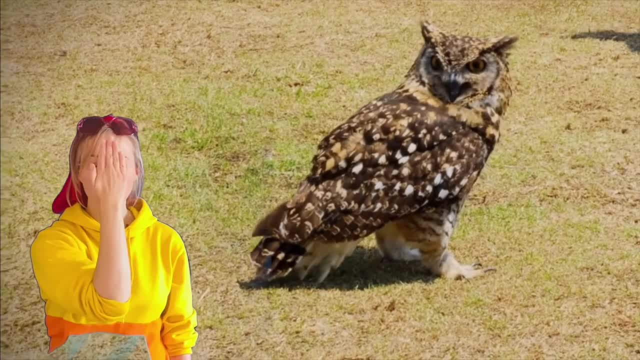 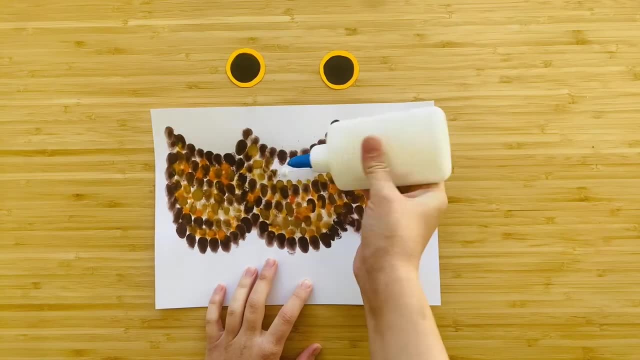 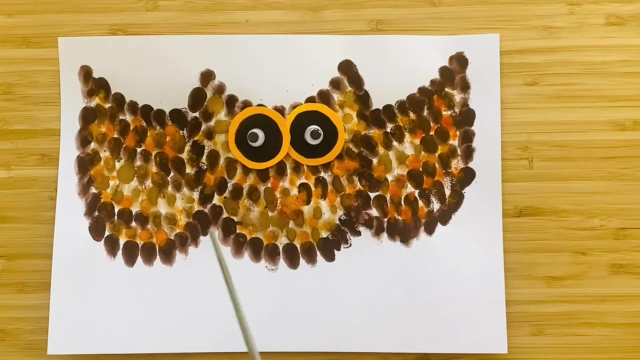 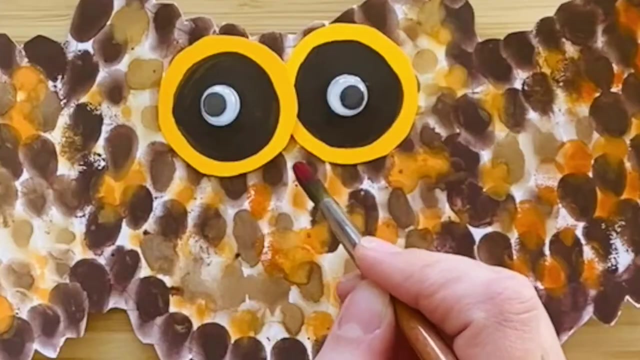 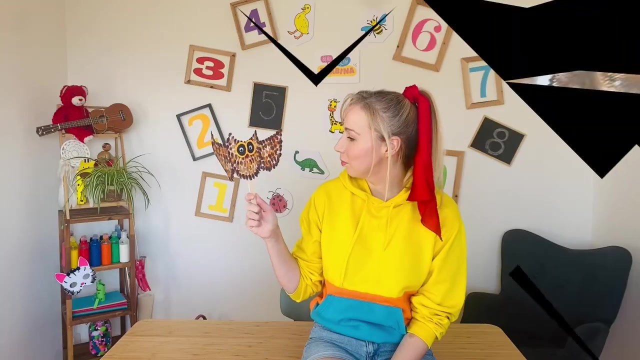 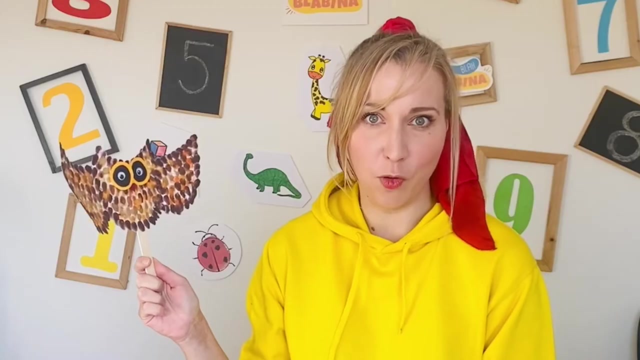 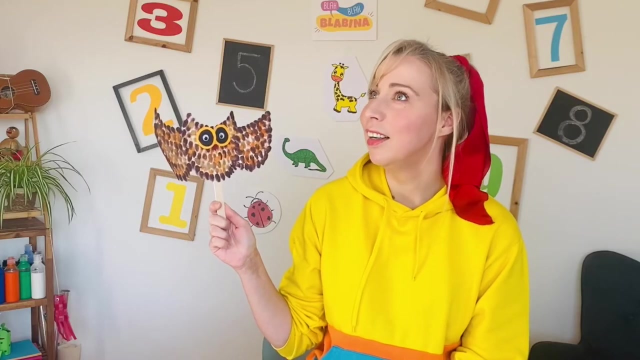 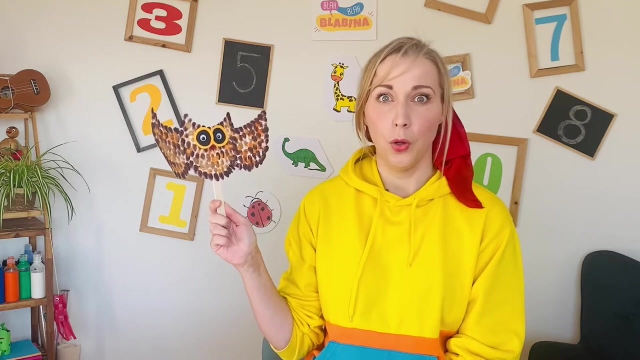 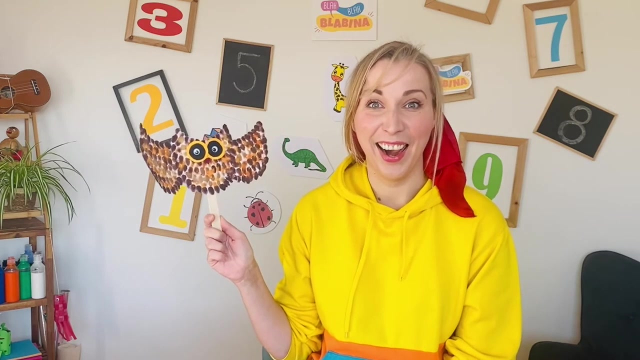 but if the Object is too close to their eyes, they need glasses. When a child is uncomfortable, they can't see, so Painless. Okay, Peter is going to teach us his language. Yes, yes, are you ready? OK, listen, OK, whee, he USB A 줄. 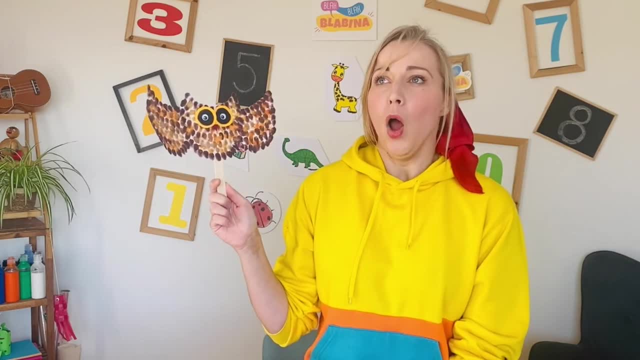 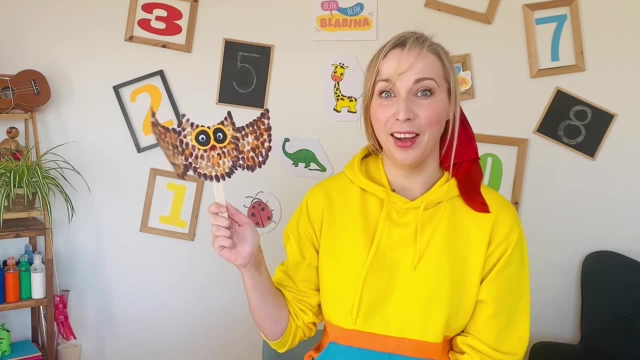 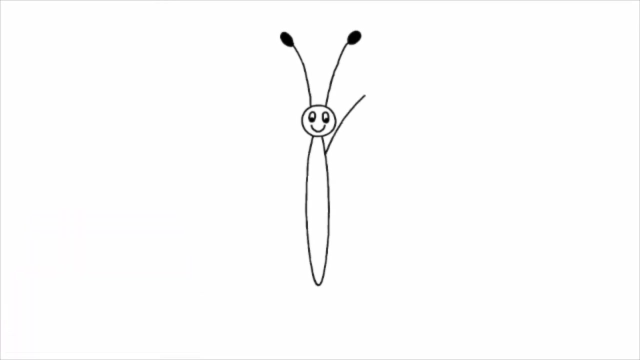 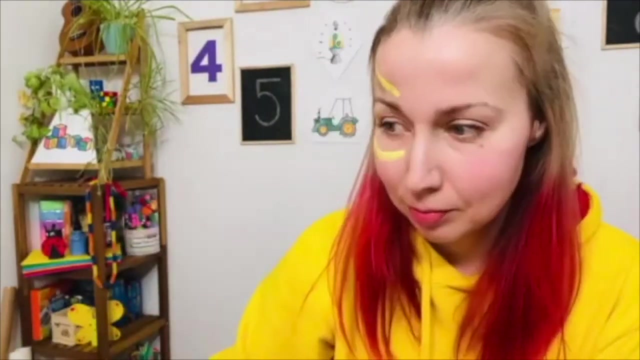 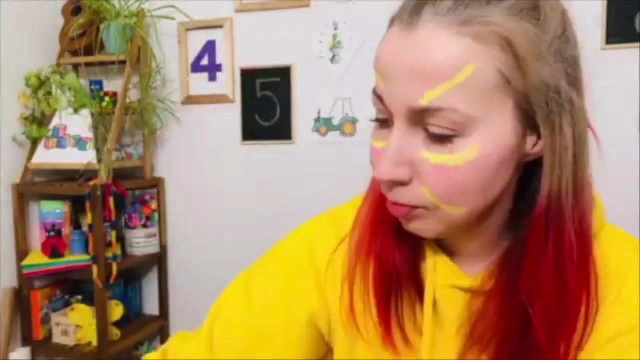 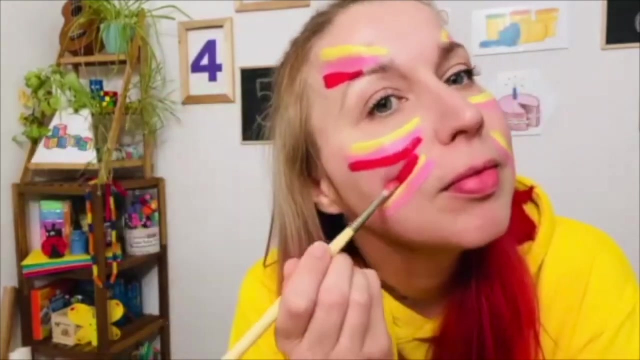 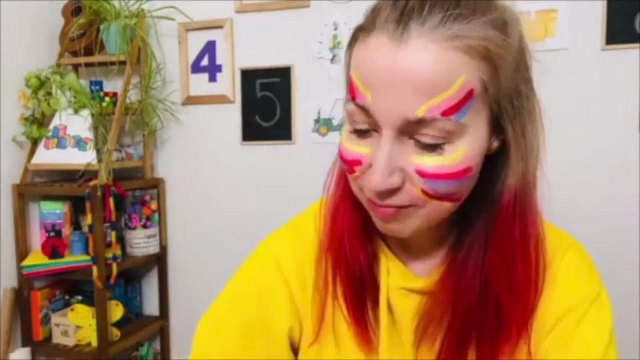 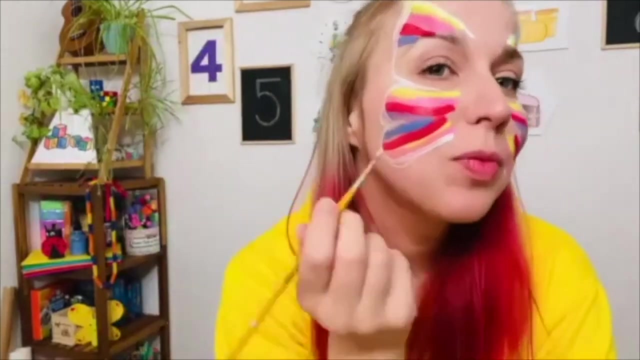 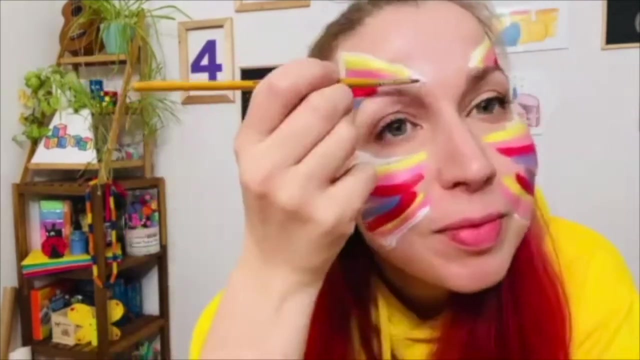 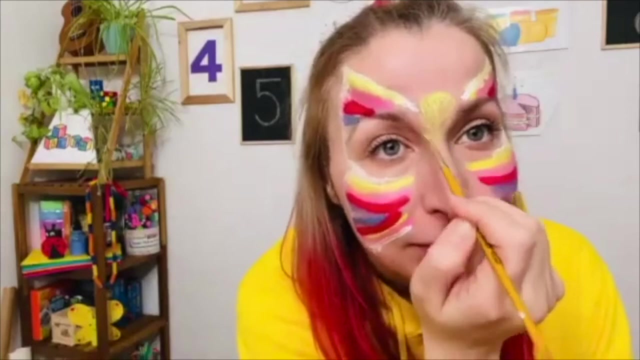 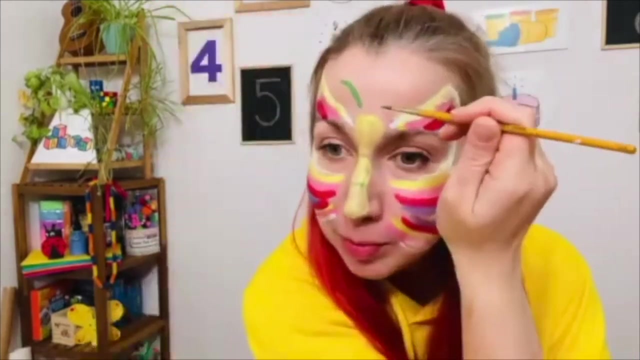 Great, Now together, Good job. Thank you Hi. I am Blabina. I love face painting. Can you guess what animal I am? Am I a frog? No, Am I a giraffe? No, I am a butterfly. 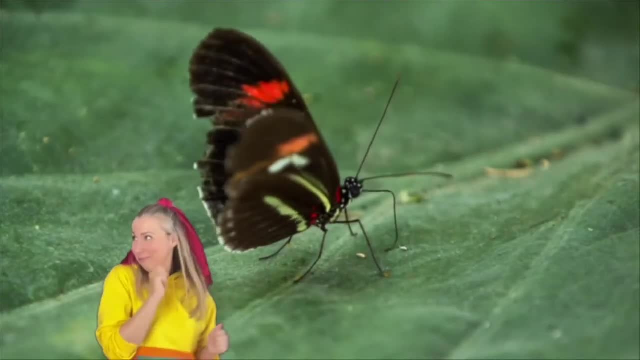 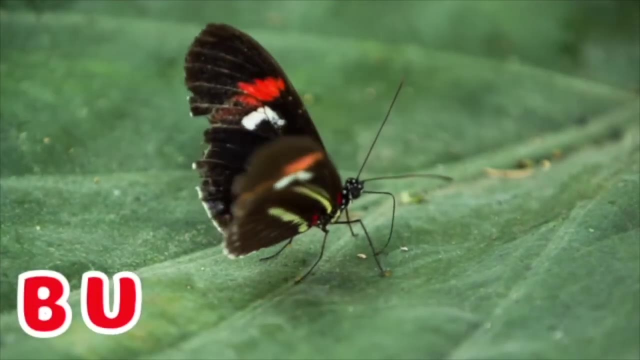 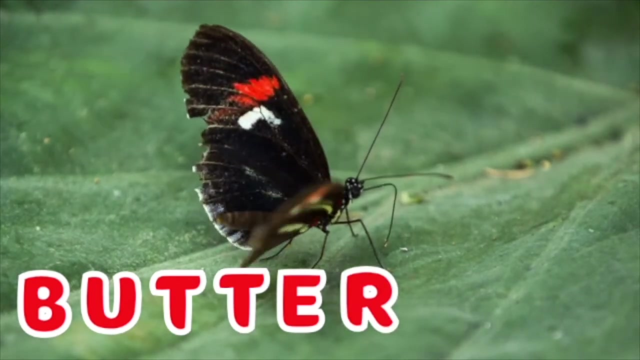 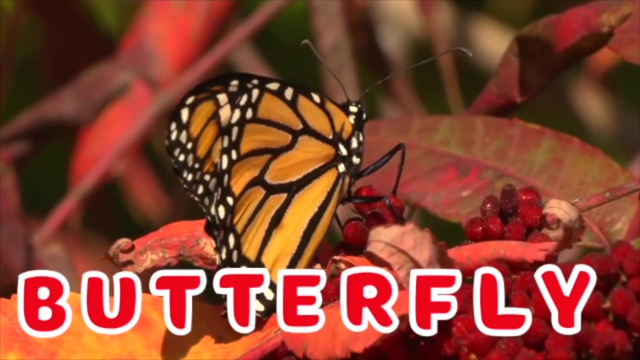 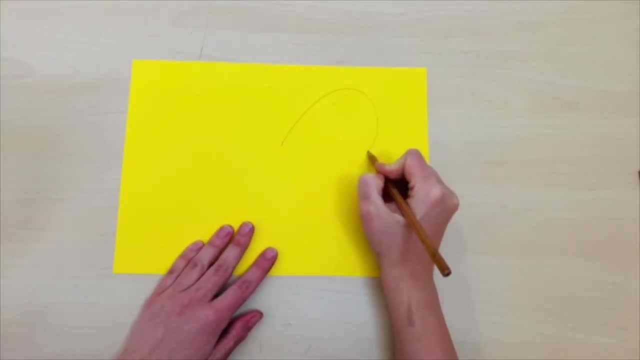 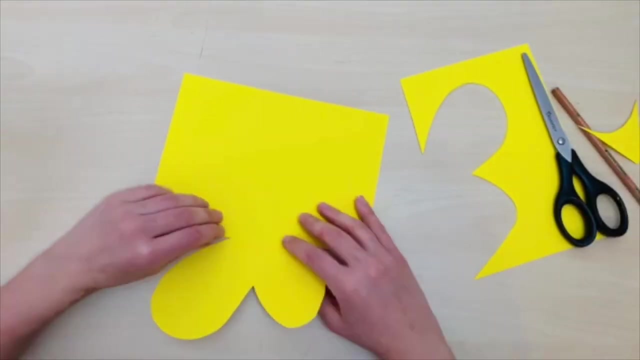 Wow, Look at this real butterfly. Can you spell butterfly with me? Let's do it. B? U T T E R, F L Y Butterfly. Good job, Hi. Can you guess what animal I am? Hi, I am a flower. 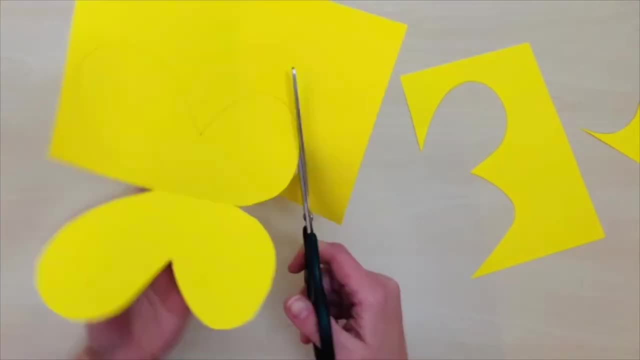 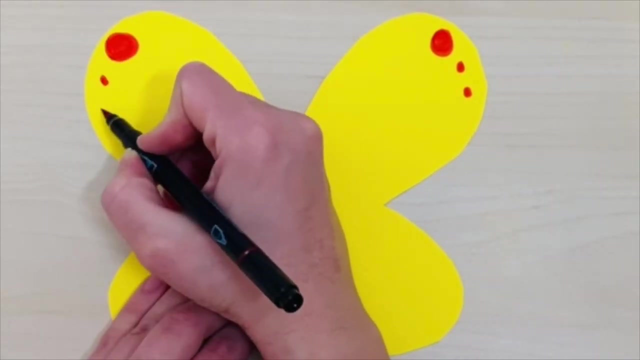 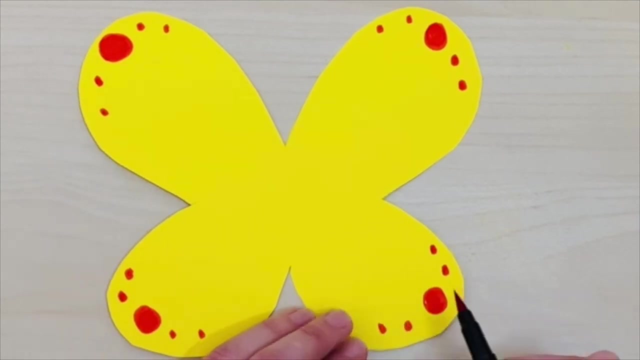 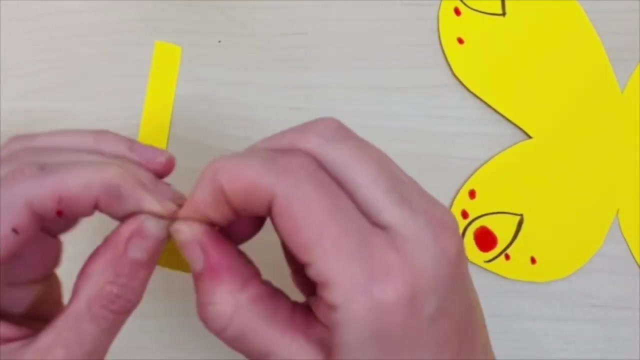 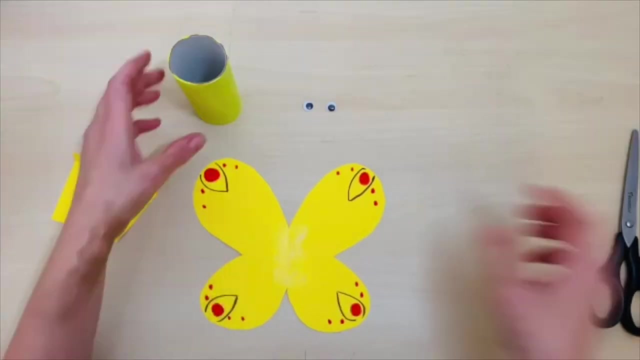 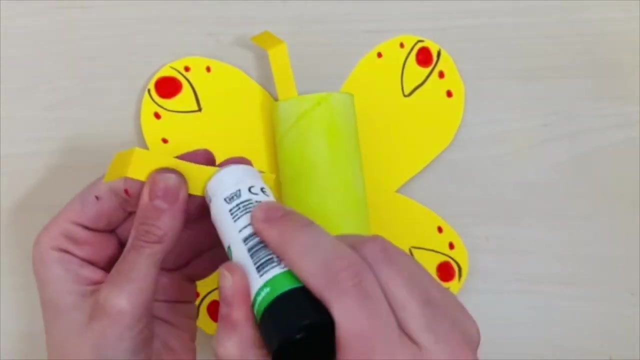 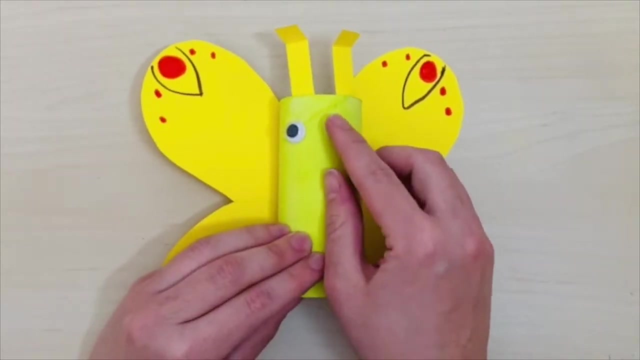 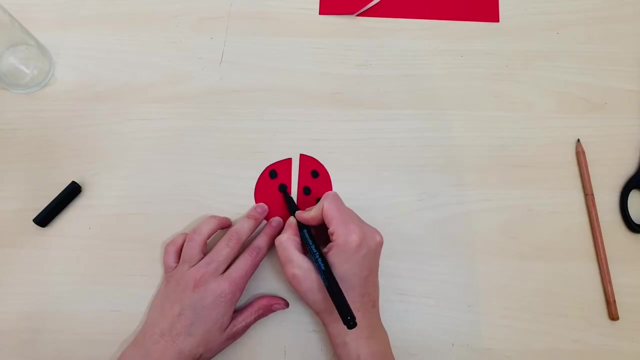 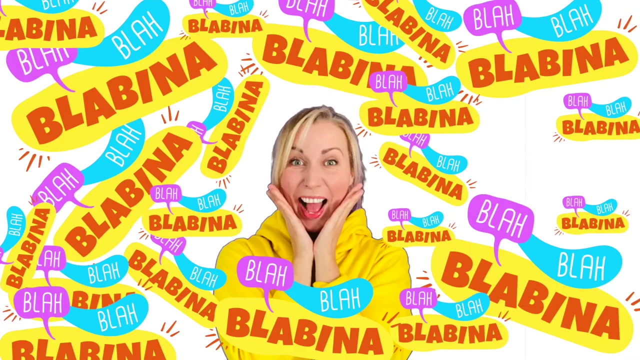 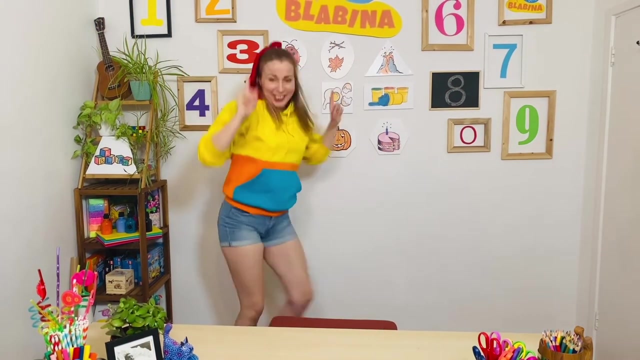 I am a butterfly, So are you. How can I guess your name? Look at this: I am a yellow dot elephant. Hi, I am a green potato. Hi, I am a red frog. We'll be right back. We'll be right back. 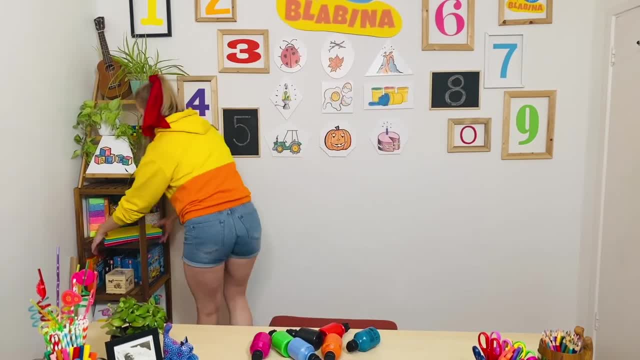 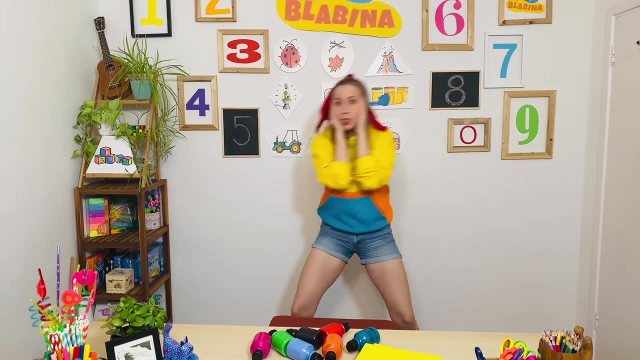 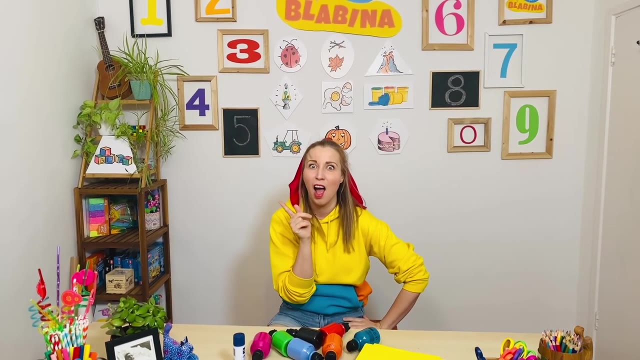 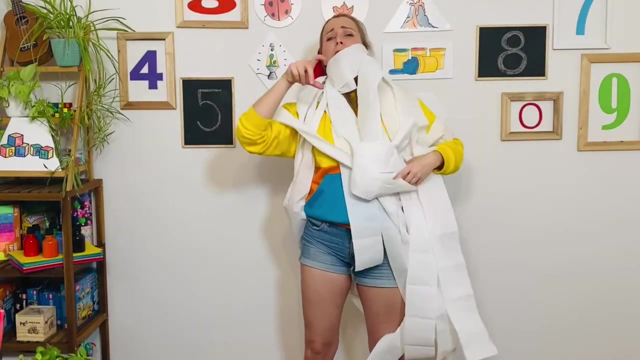 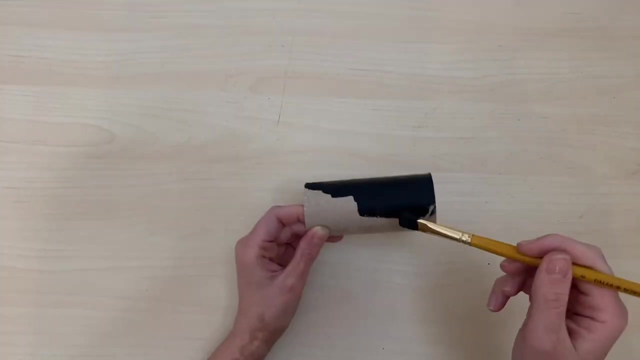 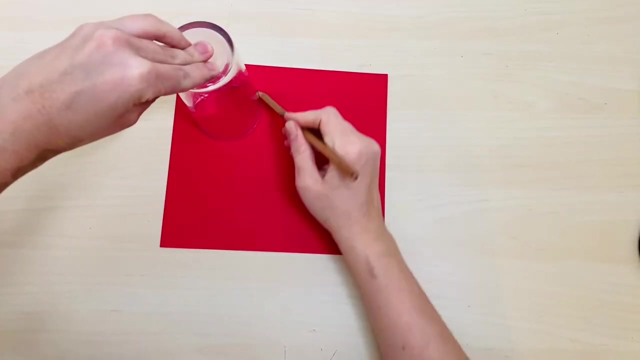 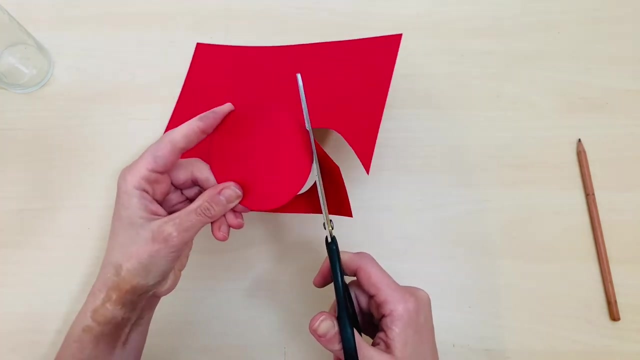 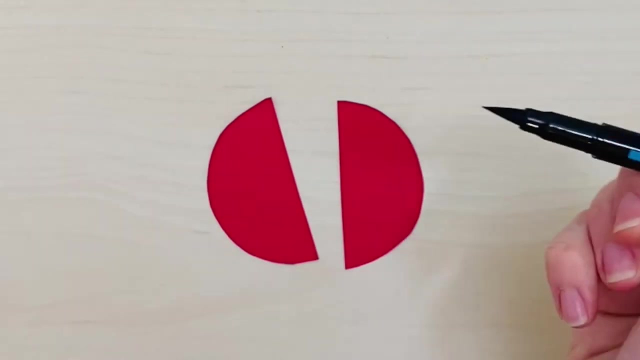 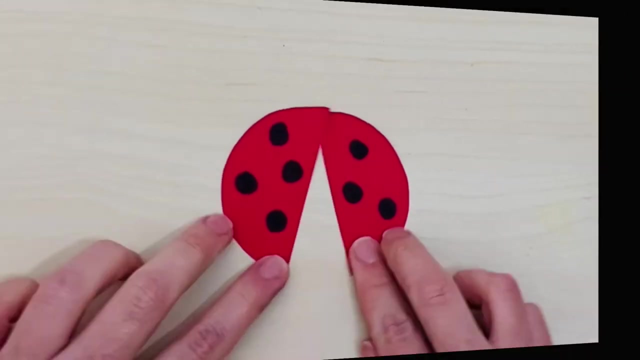 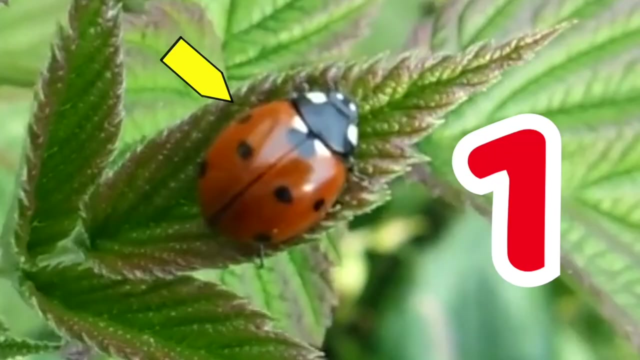 Lots of lots of paint, Then paper. We need paper, What else? Scissors And what else? Glue and paintbrush. I need some toilet roll. Black, Black, Red ladybirds have seven spots: One, two, three, four, five, six, seven.